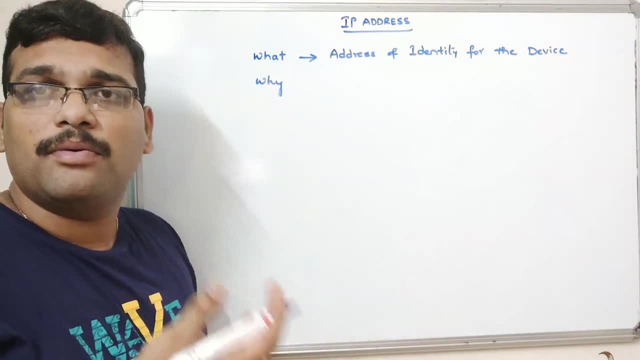 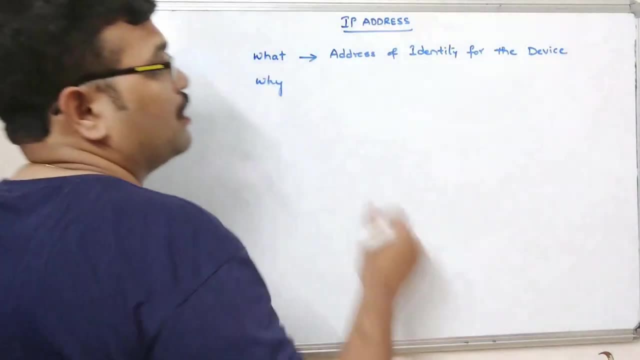 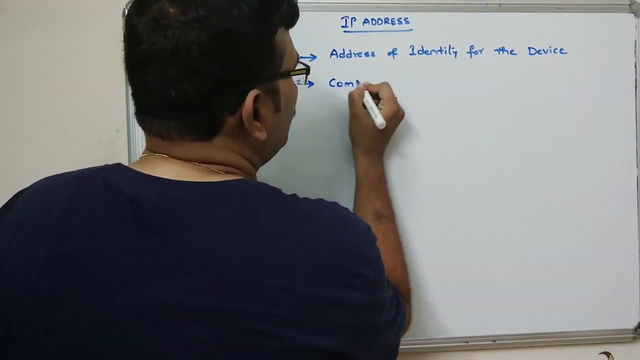 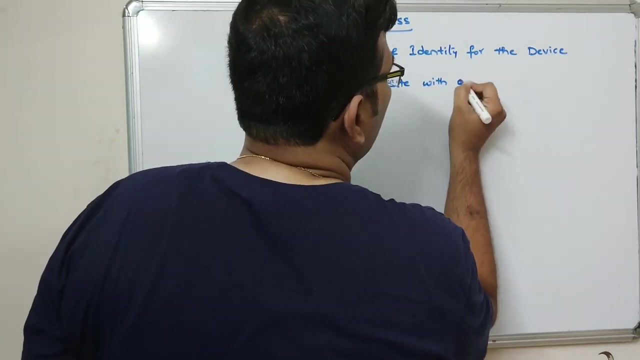 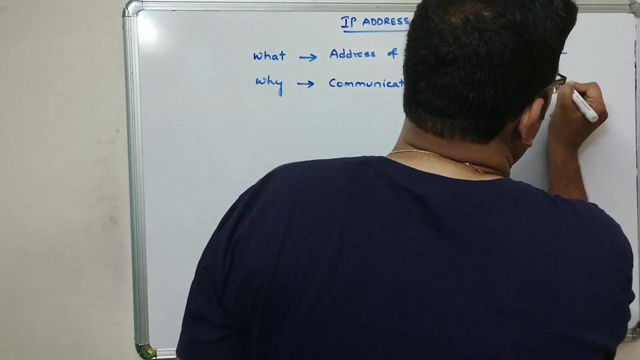 means. so it may be a computer, desktop or laptop, or a tab or mobile phone, whatever it may be. So address of identity for the device. Why? Why do we require this IP address? Simple, So the password answer is: communicate with other devices over network. So we have discussed. 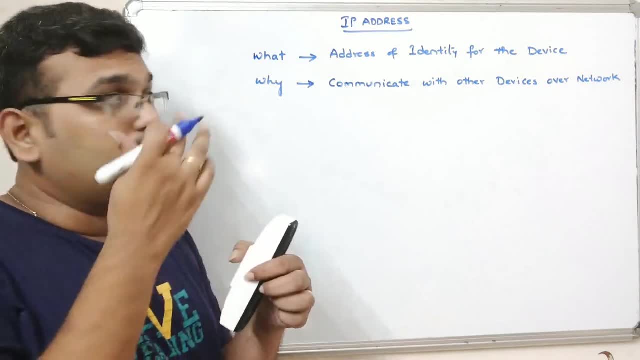 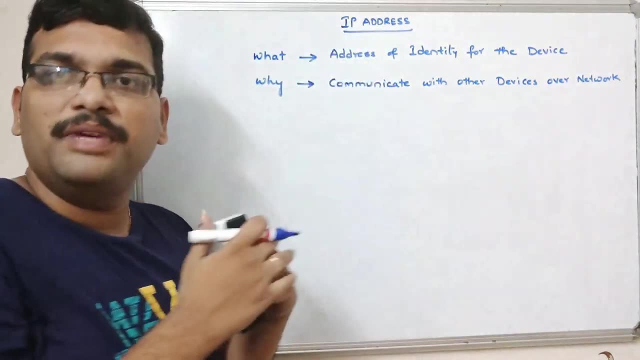 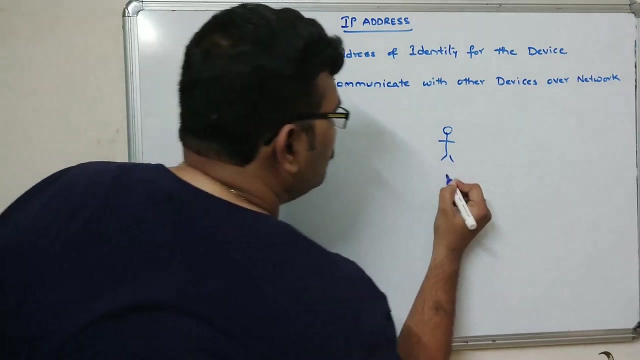 about the network. Network means a collection of all the computers, right? So in order to communicate one computer with another computer, this IP address should be required. So in this case, if you consider two persons, if you consider two persons, some A and some, 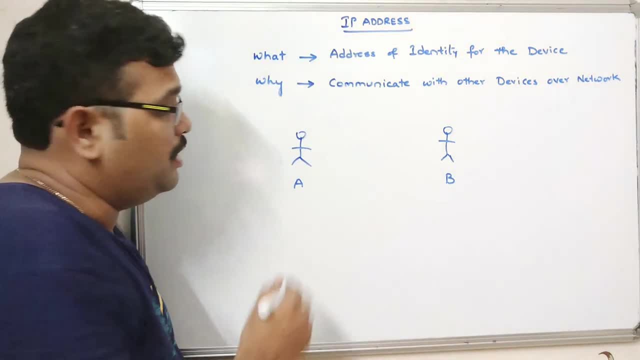 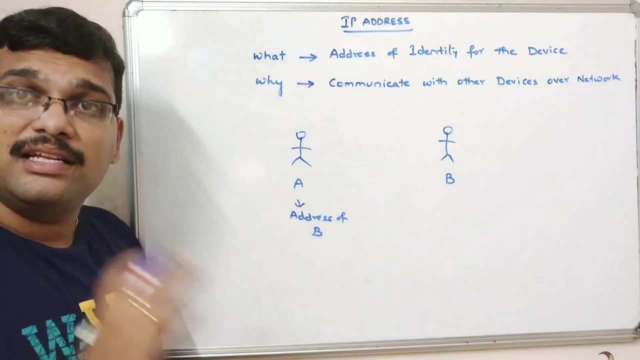 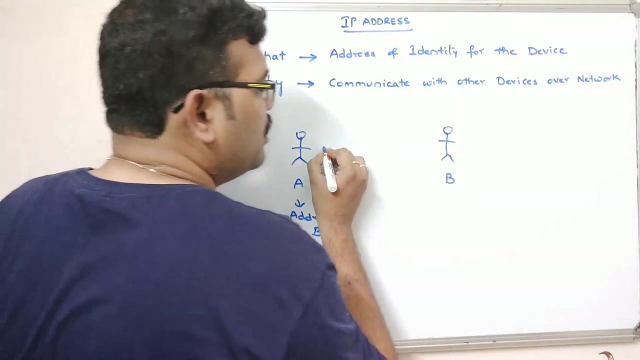 B. So if A wants to communicate with B, A should know the address of B, right? So unless A knows the address of B, A cannot communicate with B. So if A knows the address of B, then A will start communicating with the B by sending them messages. So for example, this address: 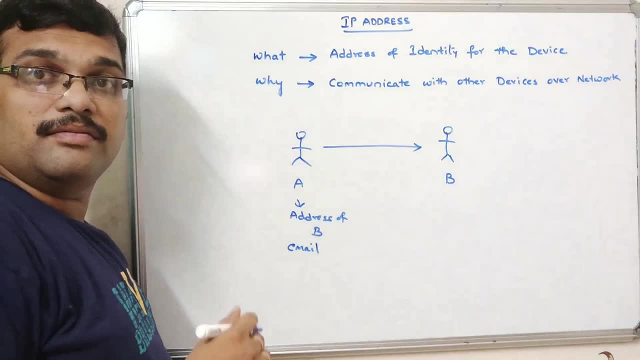 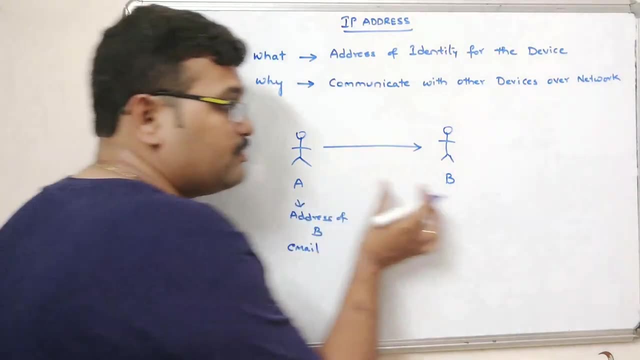 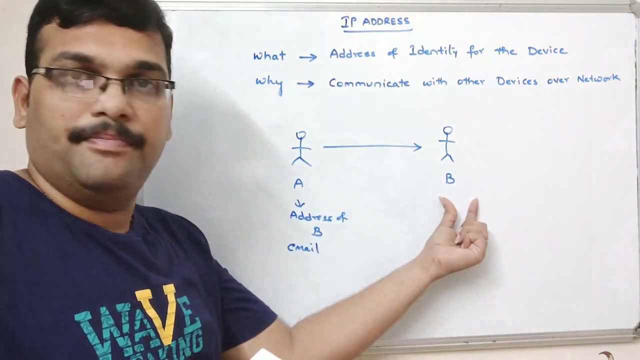 is some email Email right. So A wants to communicate with B through an email, So A should have an email address as well as B should have an email address, So A will send the message through email to the B, So A requires the address of B. that is email address right. 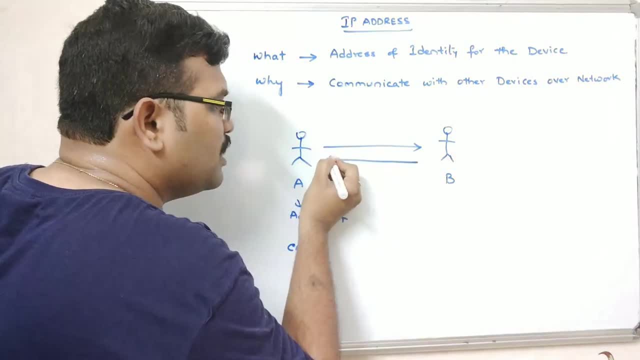 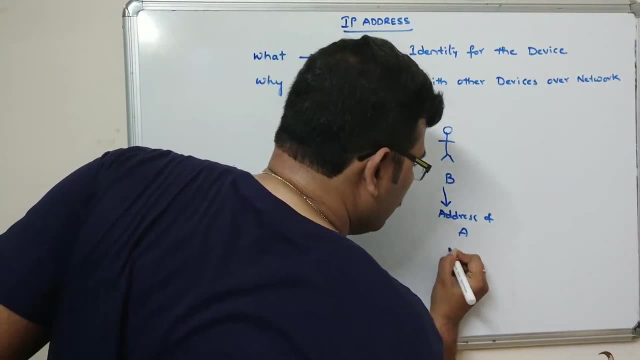 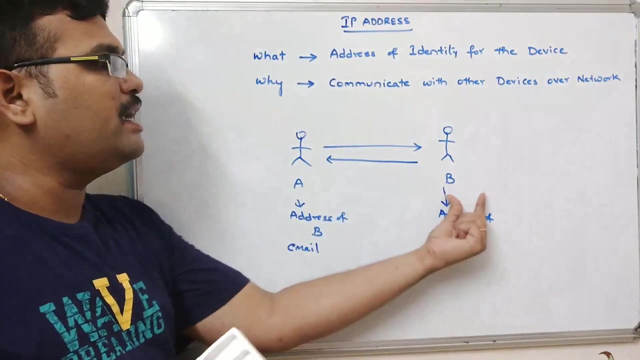 If B wants to communicate with A, B should also know the address of B. So the address of B is A right Address of A. That is nothing but email, Okay. So unless B knows the email of A, B cannot send the message. So in order to communicate between 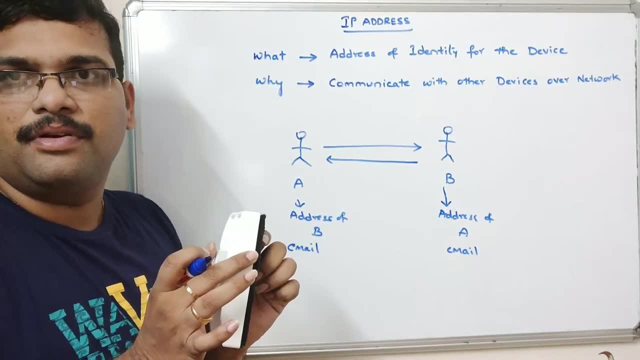 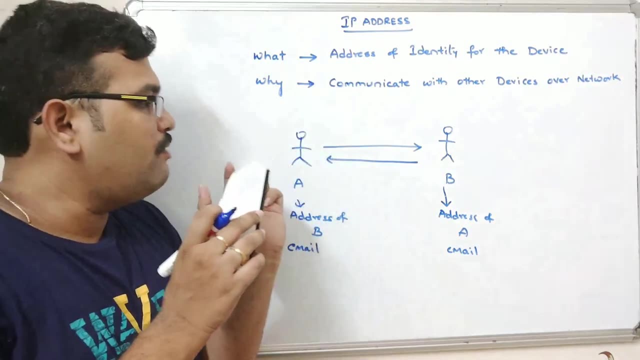 two persons, there must be some address, Right? So in the earlier days the communication will be through post, postal, right? So there will be some postal address and if A wants to communicate with B, they will write some letters and they will use the postal address. 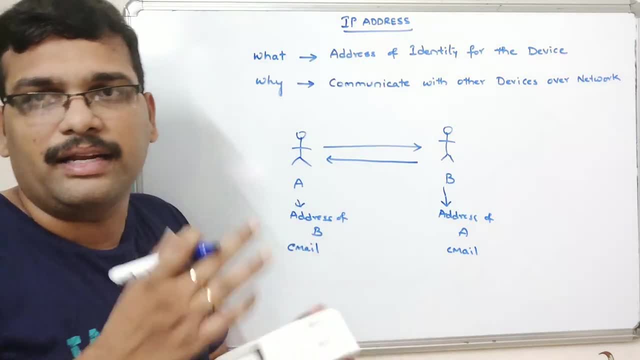 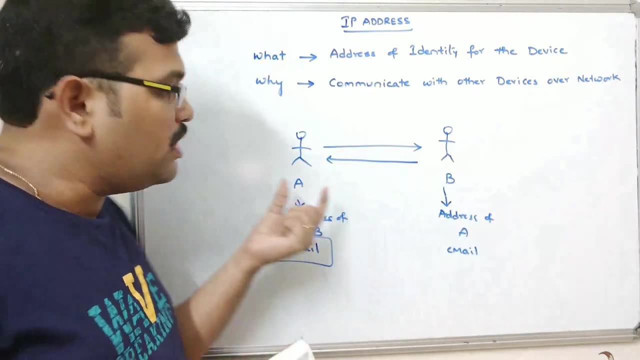 so that the message will be sent to them. So if B wants to communicate with A, B will get one email. The message will be sent via post office through the letters Right. So nowadays it's an electronic mail, So every person will be having an electronic mail. so 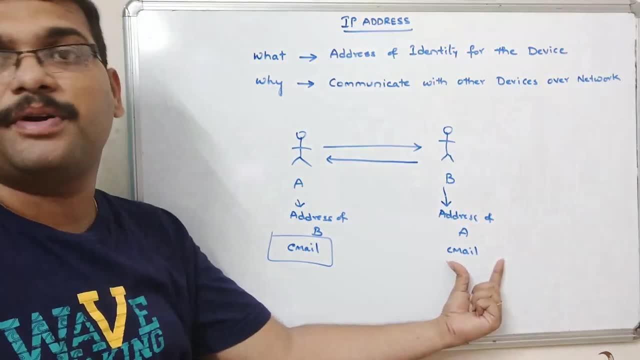 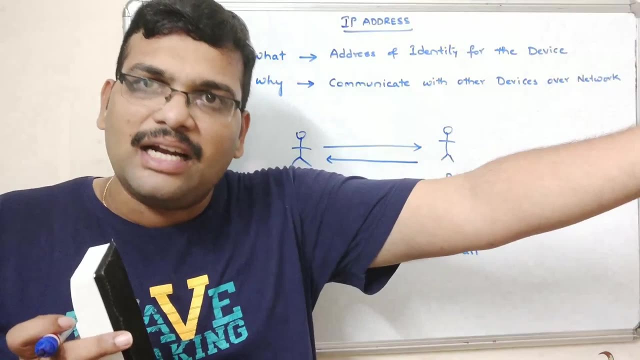 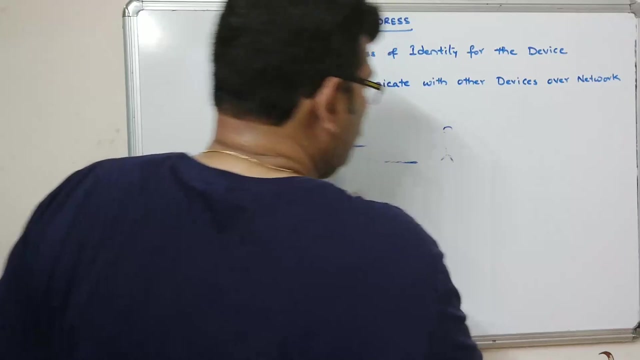 that one person will communicate with another person by knowing the address of that particular person. That means the email address of that particular person, Right? Similarly, if one device wants to communicate with another device over the network, that device should have an iPhone Right example Example. So we all know that. 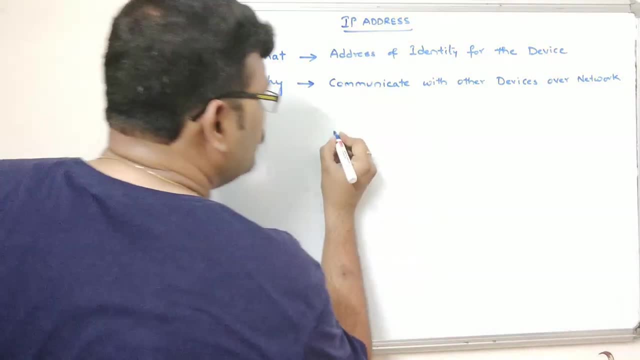 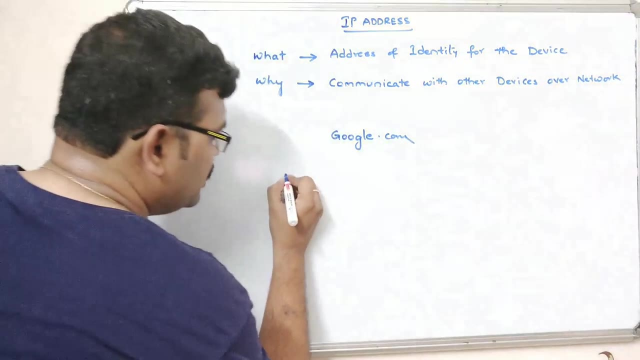 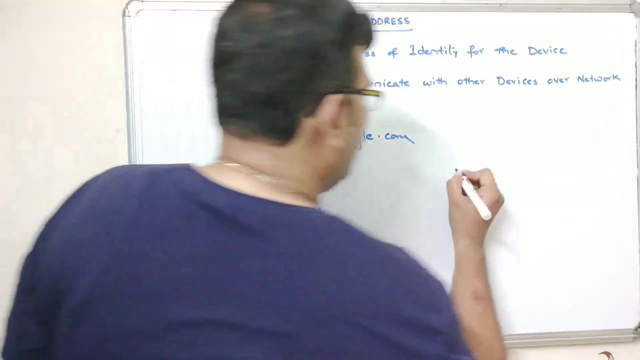 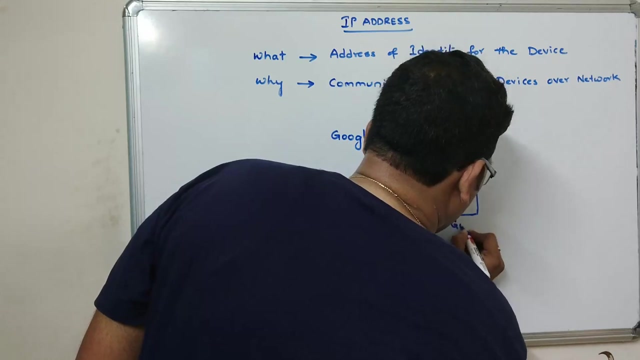 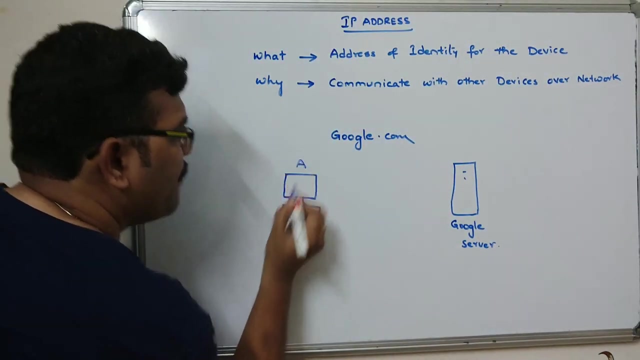 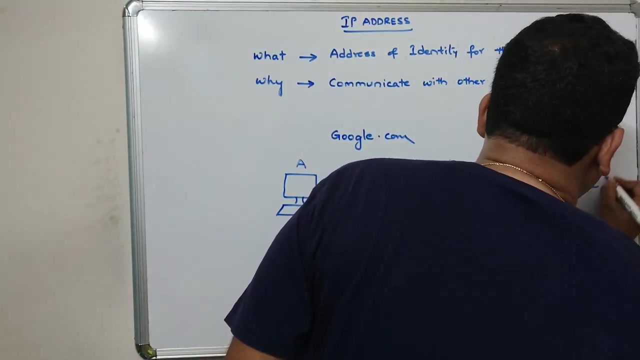 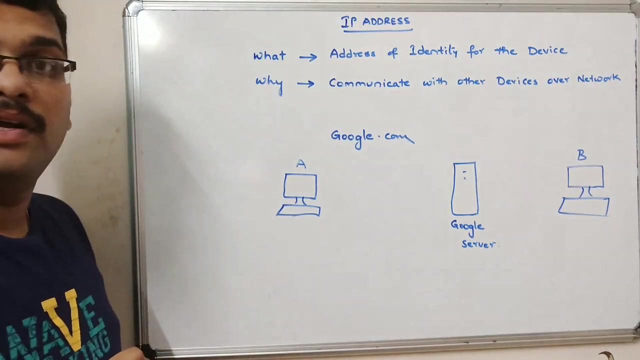 we need to know any information. the first thing we will go to be googlecom, right? googlecom. so this is my system, right, this is my system and this is the server of the Google right? so this is system A. similarly, there is a one more system in another location which is connected, so that is system B. so if A 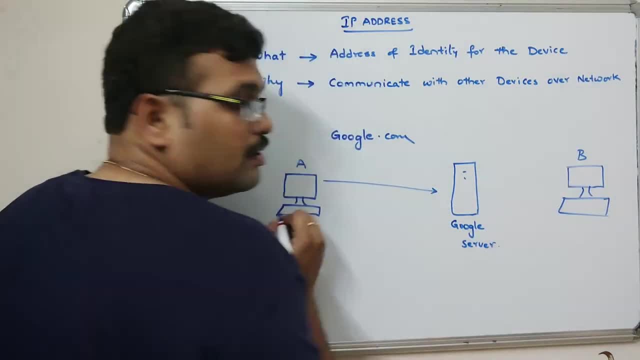 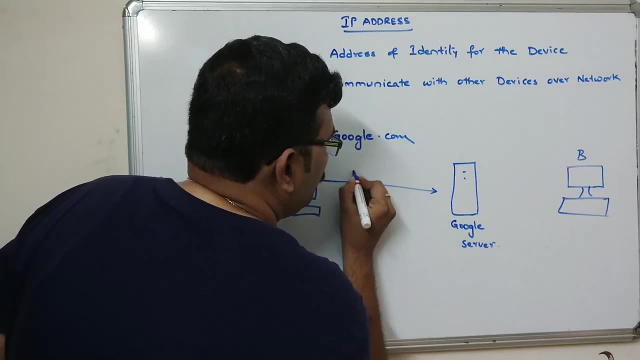 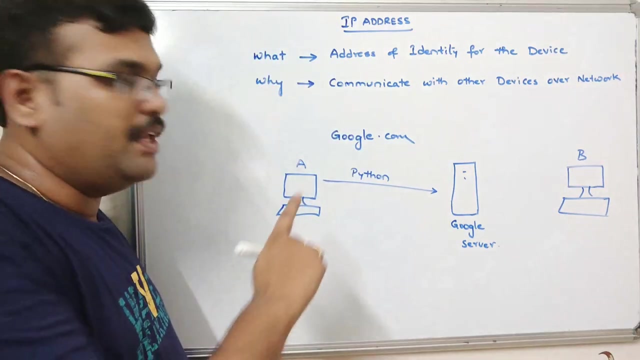 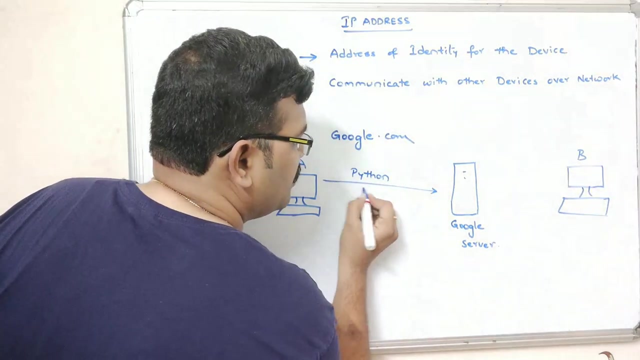 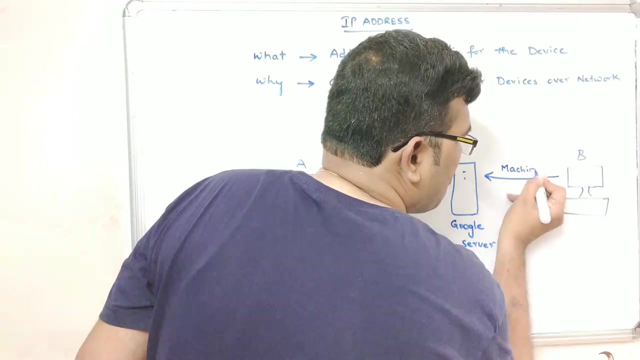 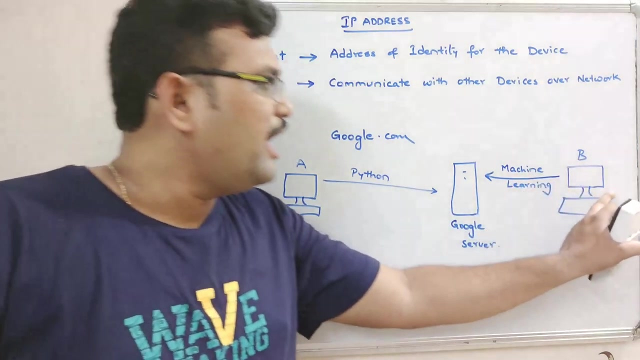 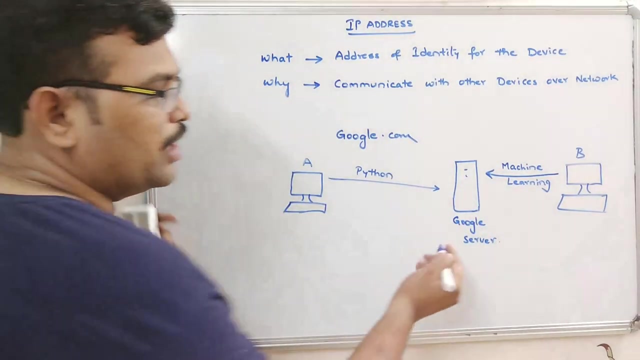 wants to search. A wants to search for for Python. okay, for Python material. simply, A will search this Python in a Google's Google server, right so Google search. and if B wants to search for machine learning, if B wants to search for machine learning, again, B also responds to this machine learning. right so now the Google server will respond to. 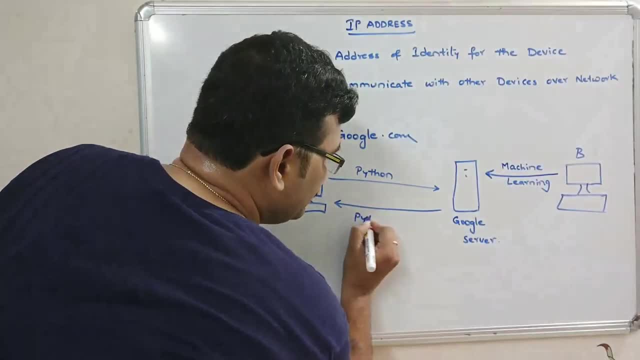 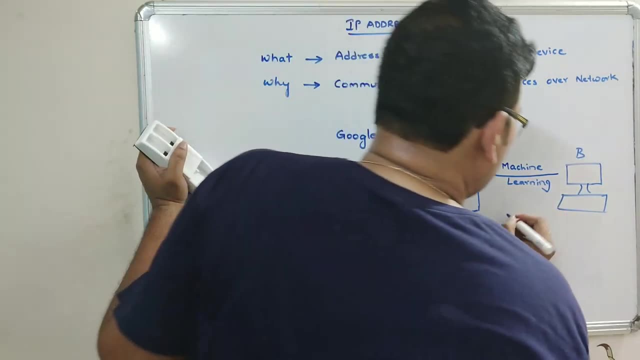 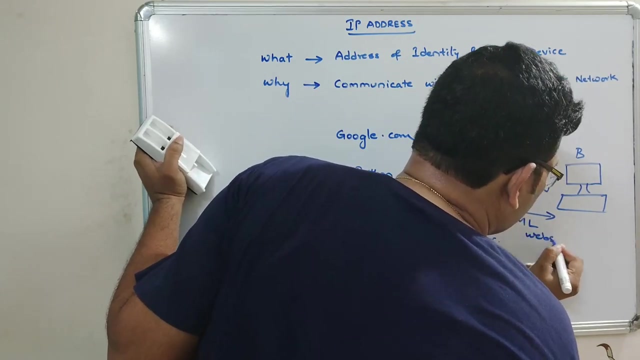 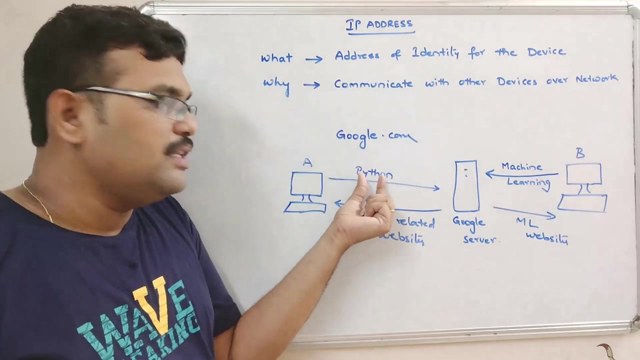 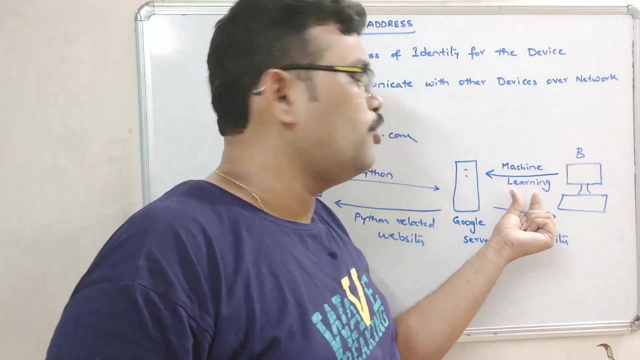 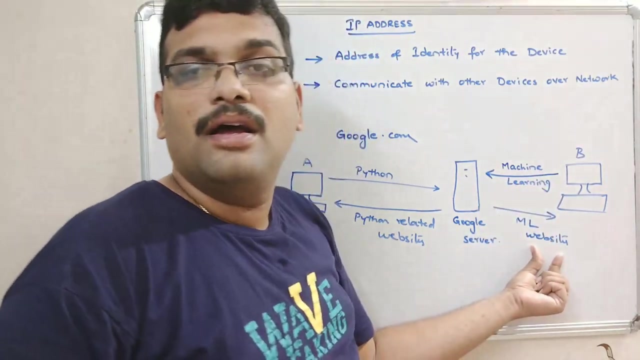 the client, so it will give some Python related websites. so this should send some ML related websites. So we all know that. So if A wants to search for Python, so automatically if you write this keyword Python in the Google search, automatically we will get some related websites. Similarly here also, If B wants to learn about machine learning, and if B use this keyword machine learning in the Google search, automatically we will get some machine learning websites. 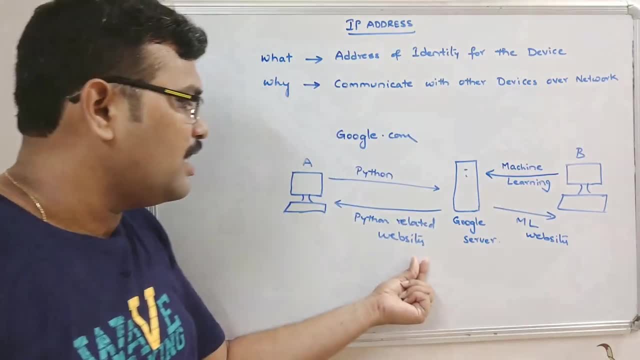 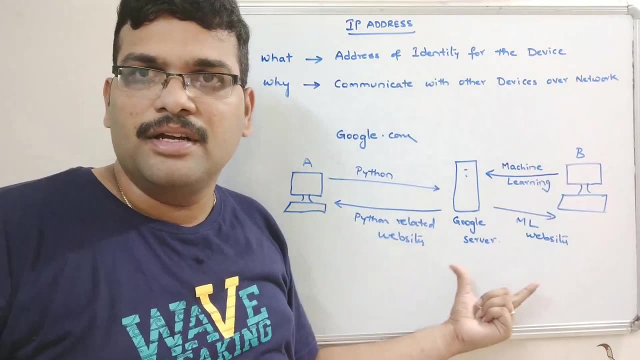 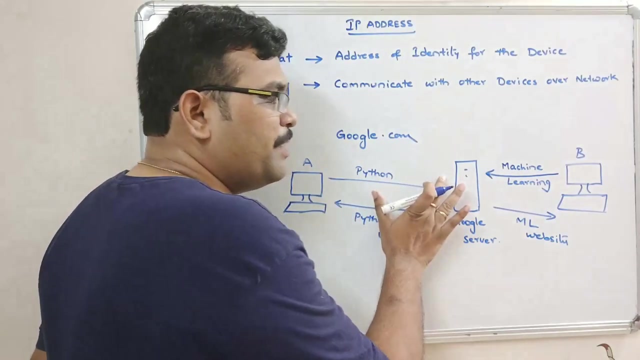 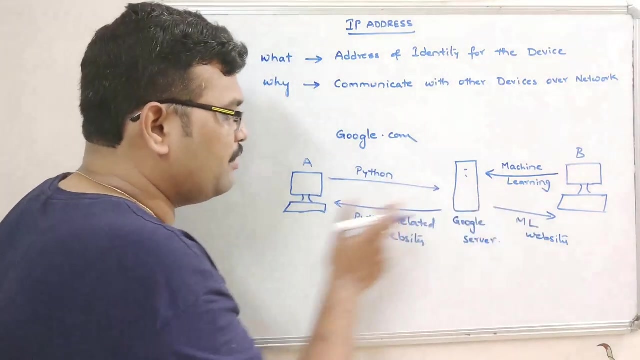 Now the question is how the Google server is sending the exact response to the particular systems. So it's a single server maintaining all the systems. So it's giving response to all the systems, Right? So A is sending some Python keyword and the server should respond to that system itself. So Google should not send the machine learning websites to A and Google should not send the Python related websites to B. 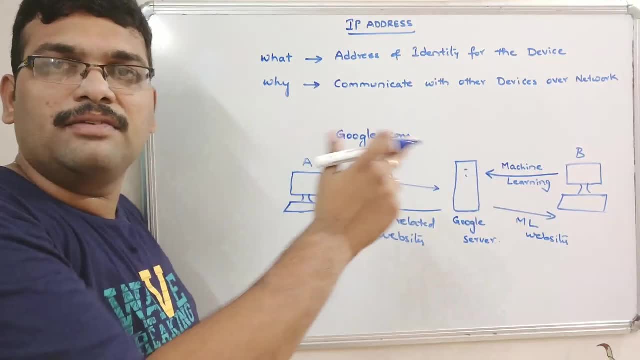 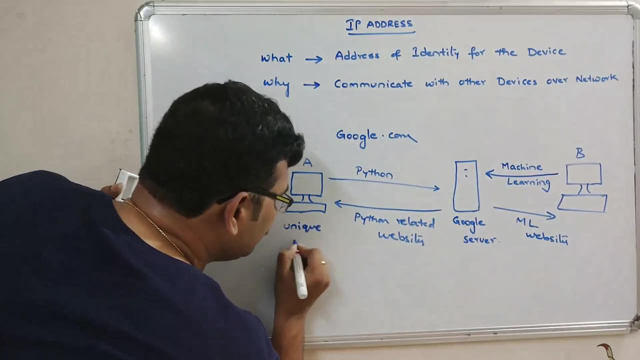 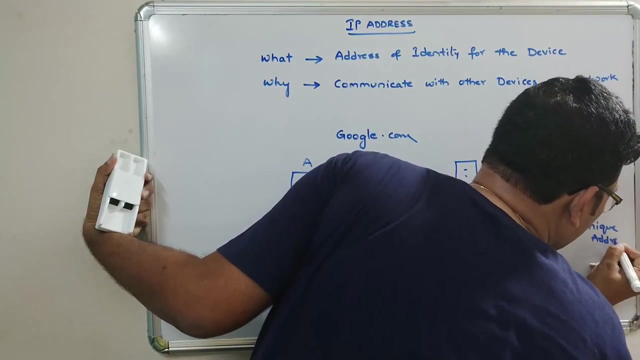 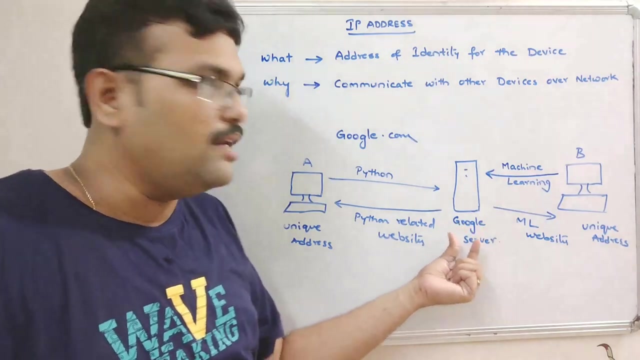 Right. So this proper communication will be done only through the address, the unique address. So A will maintain some unique address. Similarly, B will maintain some unique address. So, based upon this unique address, if A sends the Python keyword to Google search, automatically that Google server will send the response as a Python related websites to the address. 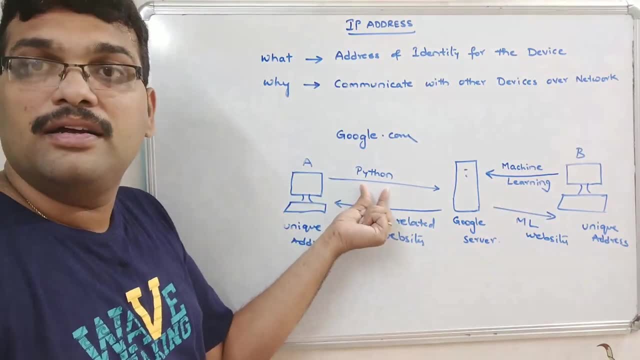 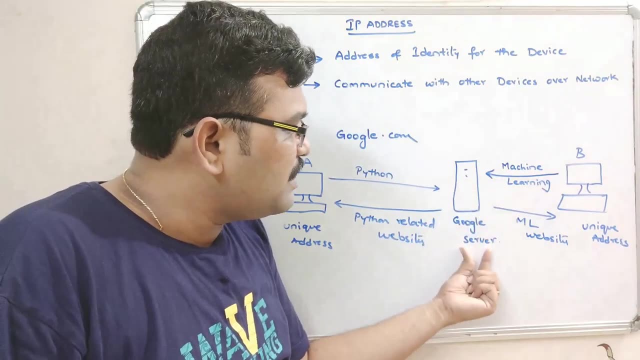 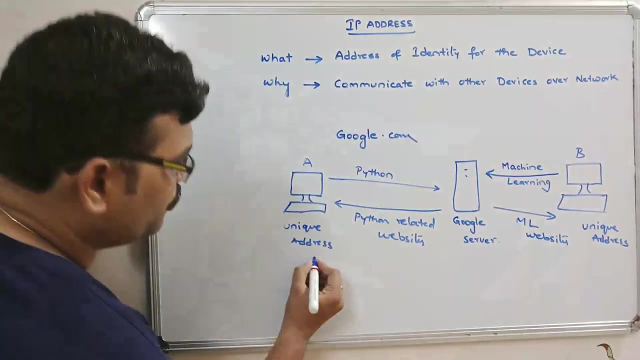 So B will maintain some unique address, unique address from where it received the request. Similarly B. if B sends the request of machine learning keyword, so Google Server will send this ML websites as a response to the unique address of B. So this unique address we call as IP address. 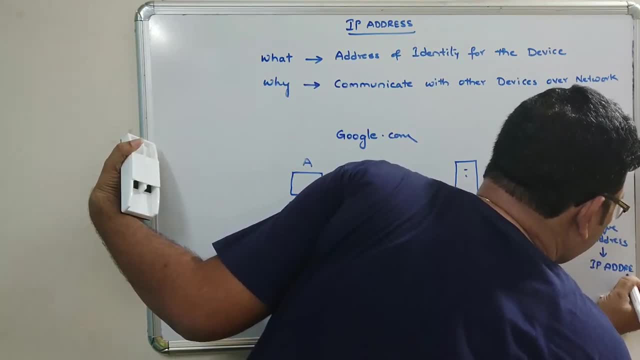 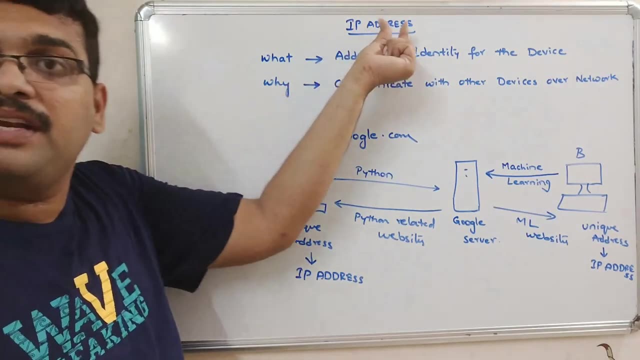 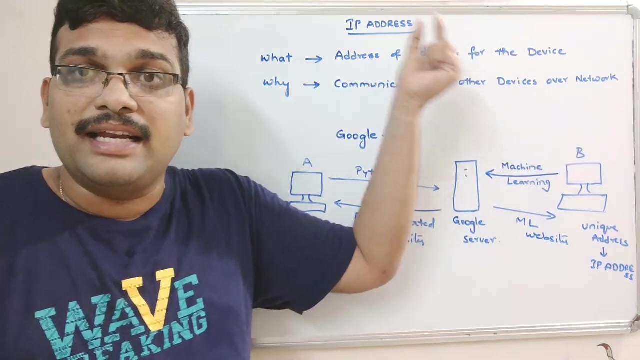 This unique address is called IP address. So that's why I am saying why. why we need this IP address means communicate with another devices, other devices over network, So it's an internet. in the internet there would be a large number of computers. 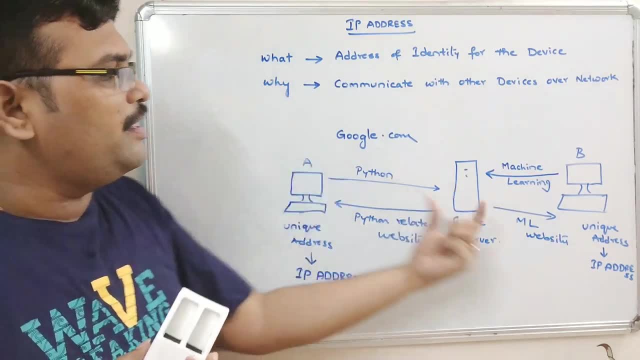 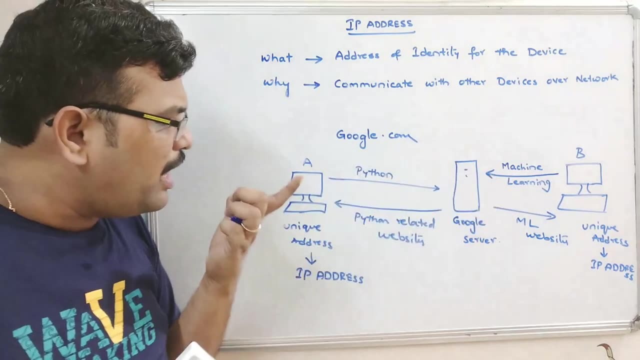 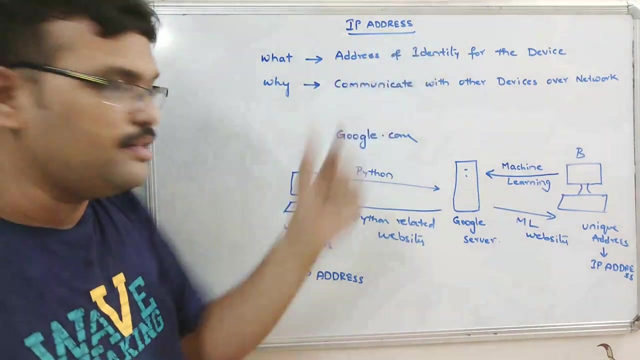 So interacting one another right. So it will interact with the server, it will send the request to the server and it will get the response from the server. So everything, every communication in the internet, will be done with the help of this IP address. 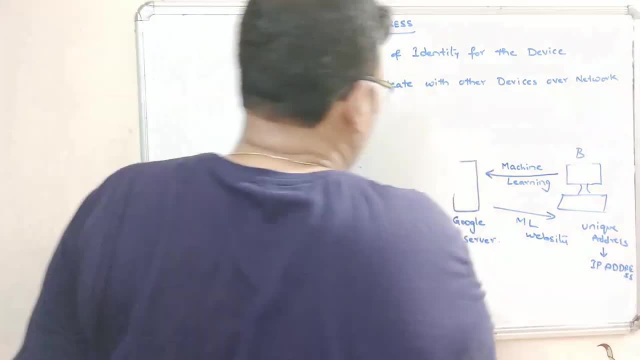 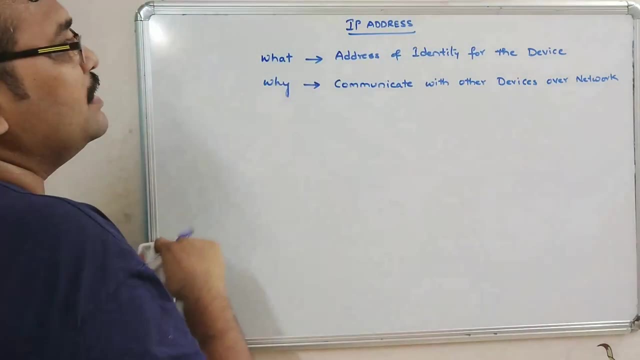 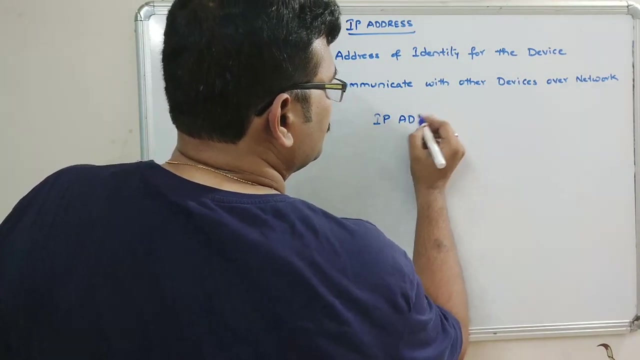 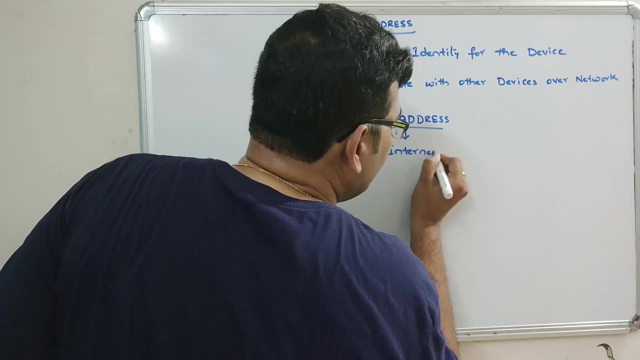 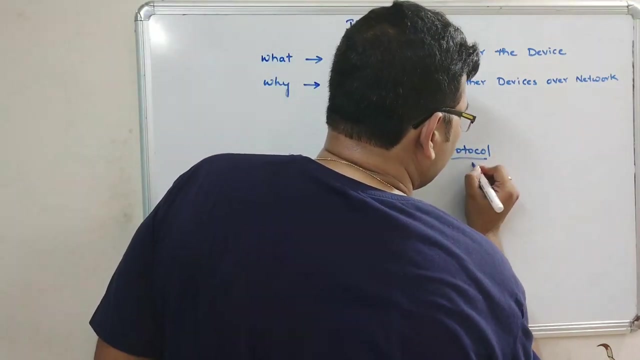 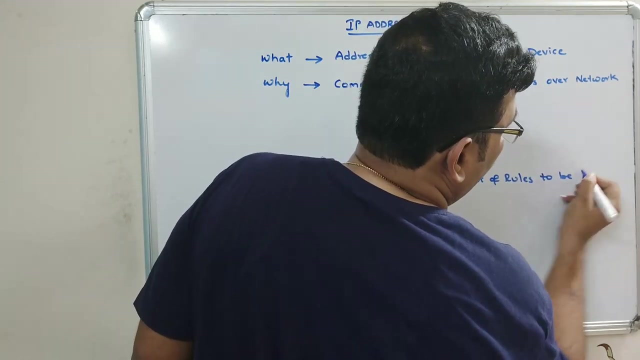 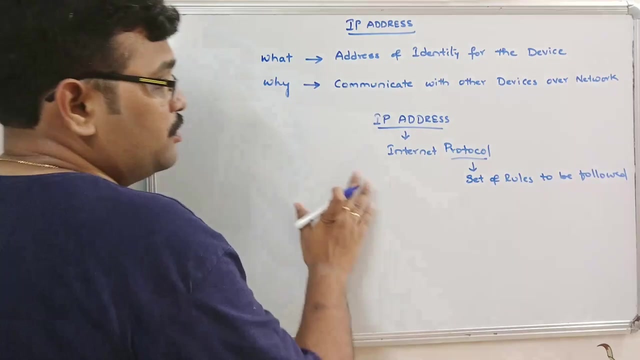 So hope you understood this basic thing Now. IP address means internet protocol address, internet protocol, internet protocol. So here the protocol means some set of rules to be followed, some set of rules to be followed, right? So this IP address will be having in the form of four format: 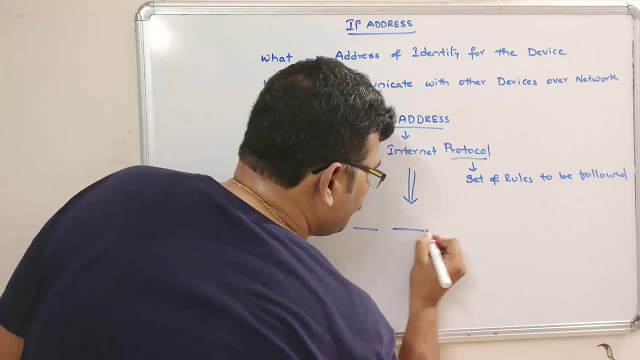 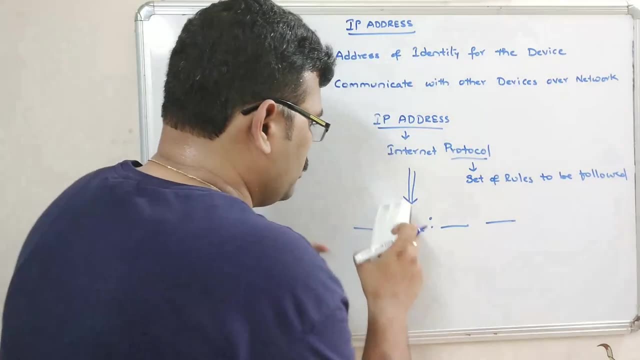 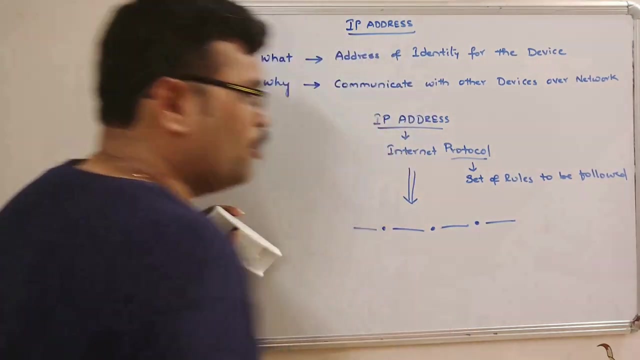 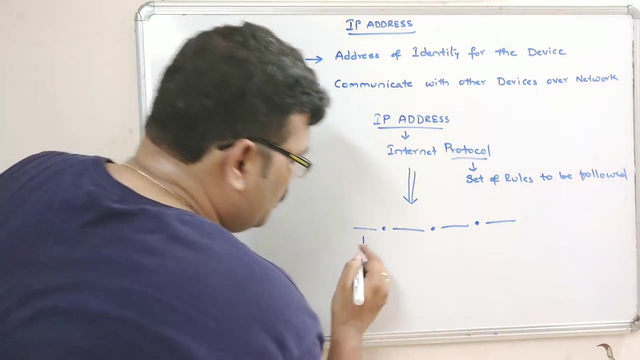 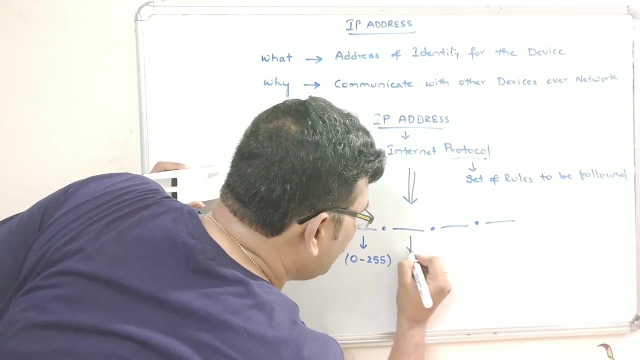 So the IP address will be having in the form of four format and the IP address will be following the IP address formats: four parts separated with a dot and each part will be having the numbers from 0 to 255.. And this part will also be having 0 to 255.. This will be also having 0 to 255,. 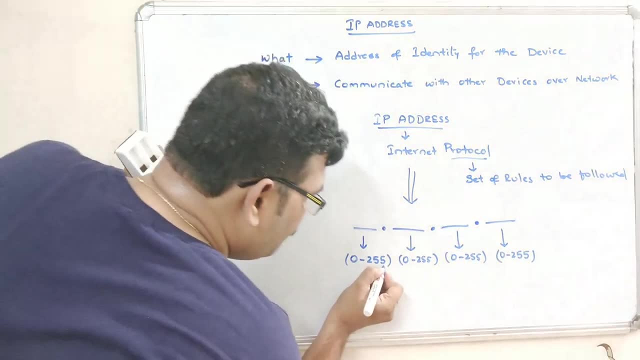 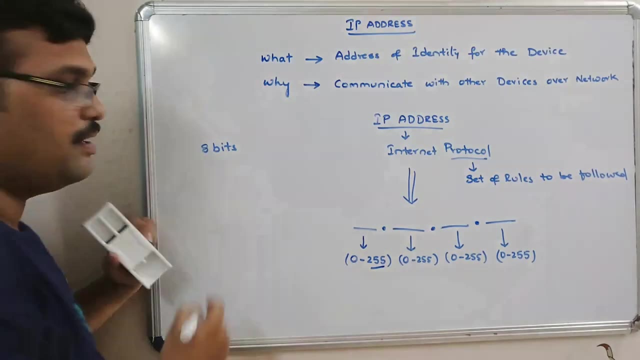 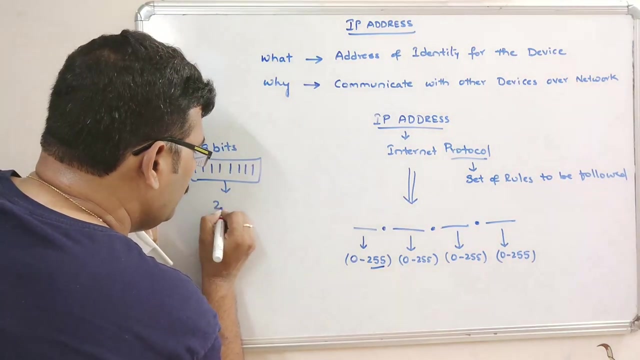 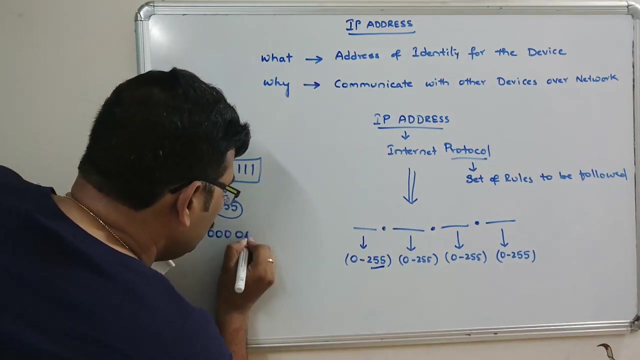 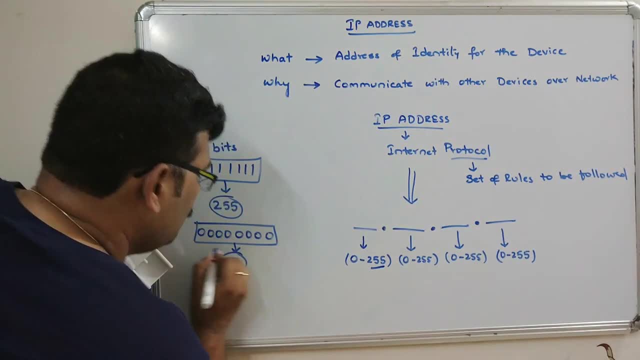 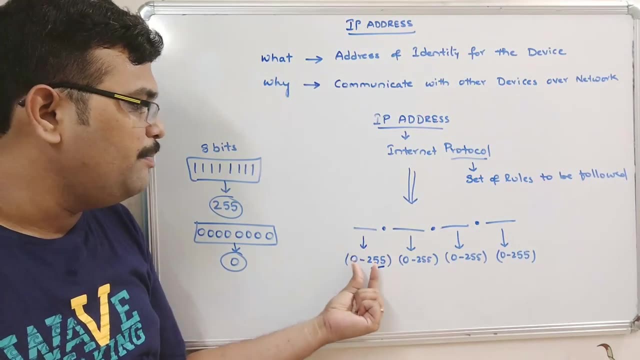 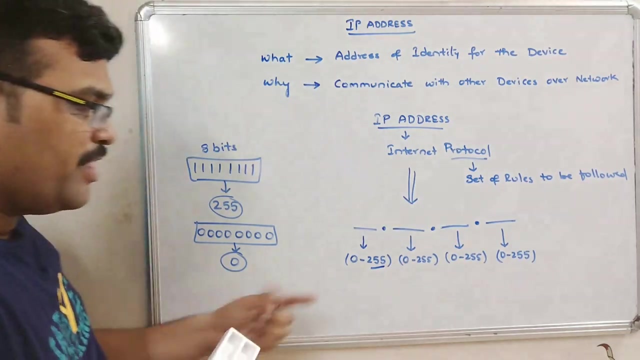 represents the decimal value 0. so for every section, so there will be 4 sections, so for every section it will be filled with one number among 0 to 255, ranging from 0 to 255, and so so we know that the system doesn't know these decimals and all these things. only it can. 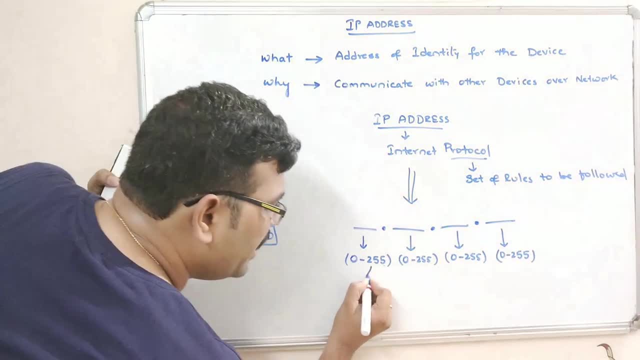 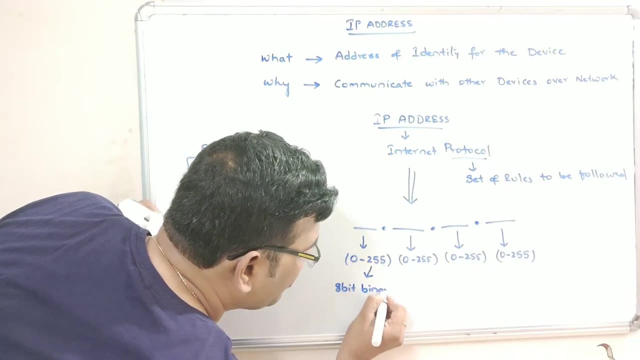 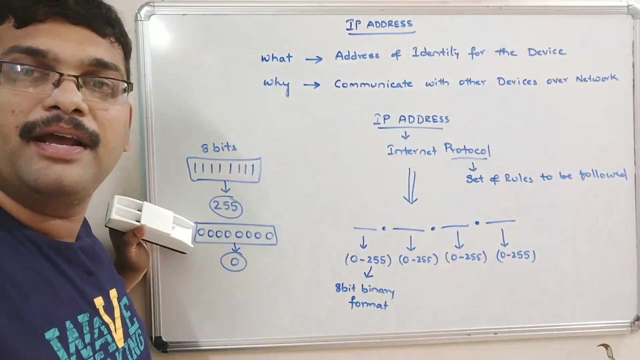 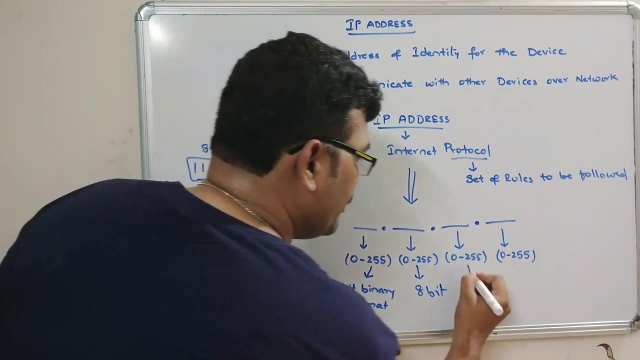 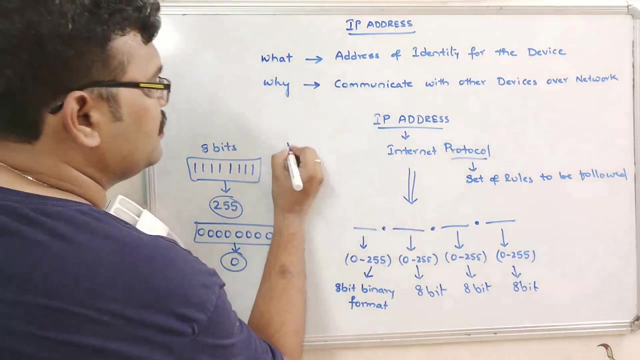 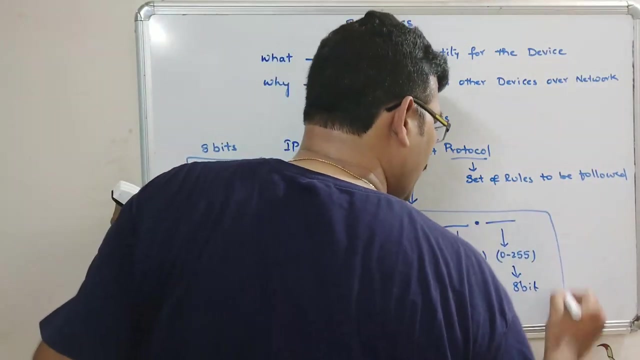 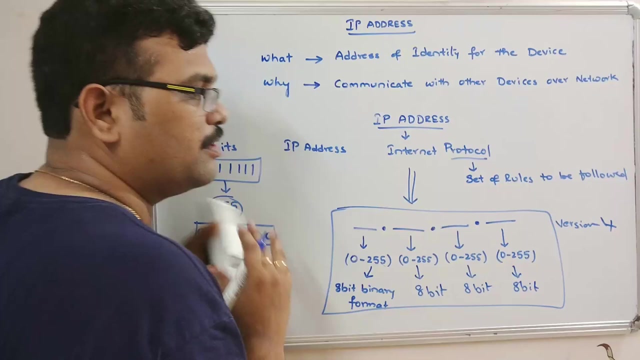 understand the binary numbers, right. so that's why this will be again converted into 8 bit binary, 8 bit binary format, 8 bit, 8 bit binary format, 8 bit binary format, right, and similarly, here also, we'll get 8 bit. here also, we'll get 8 bit. here also, we'll get 8 bit. so the IP address- so I mean IP address and all these- is in version 4, so there are different versions, right? so 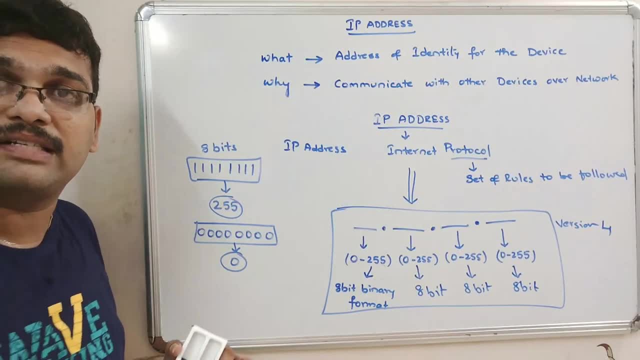 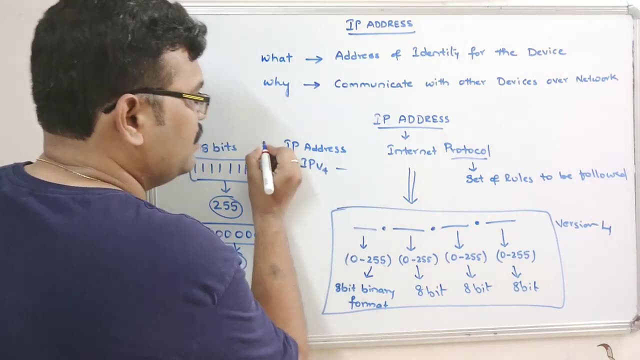 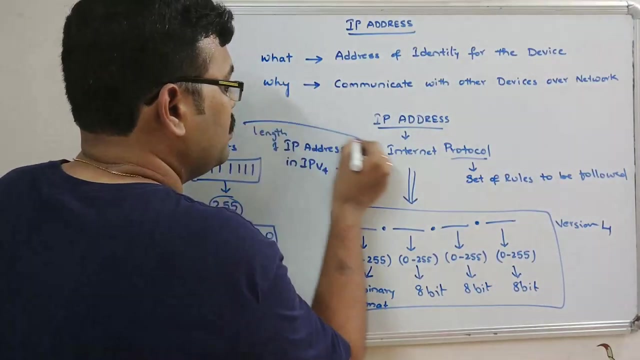 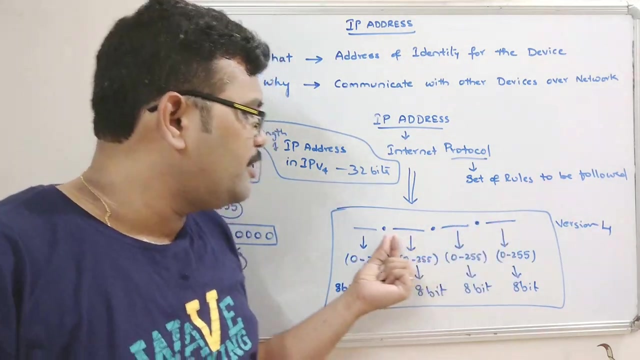 this is for IP version 4. okay, IP version 4. so IP address in IP version 4 is the length, the length. okay, the length of IP address is 32 bits. right, the length of IP address in IP version 4 is four sections divided with the dot, and each section is: 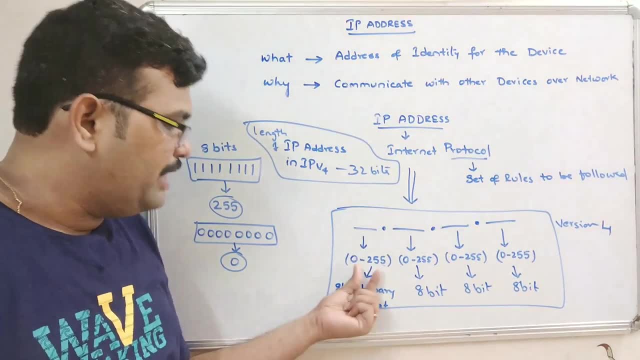 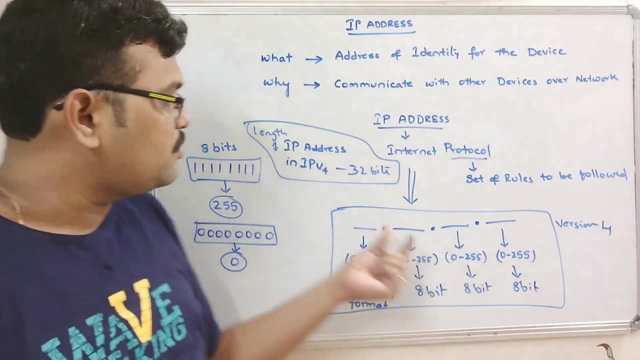 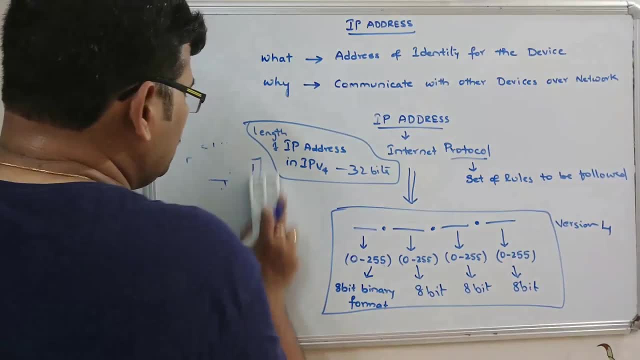 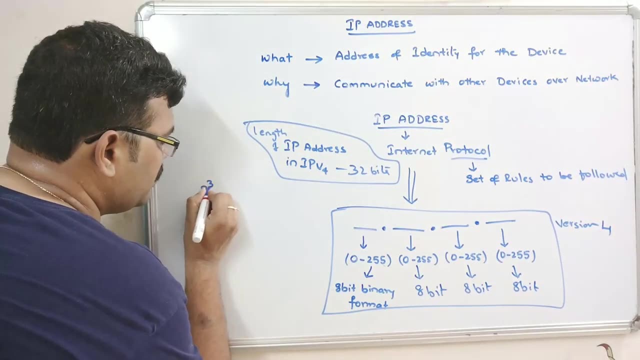 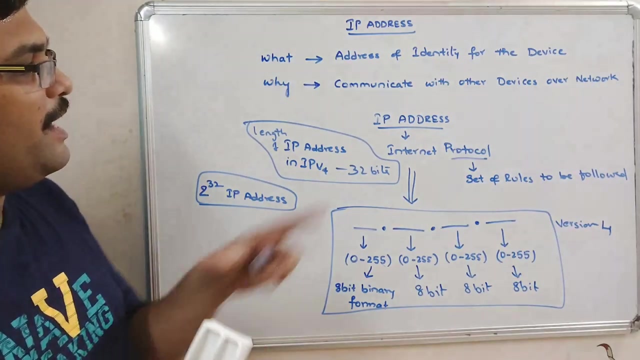 So it represents 32 bits And see from these 32 bits how many IP addresses can be generated. So 2 power 32 IP addresses will be generated. So why I am saying this? is this IP address should be unique. 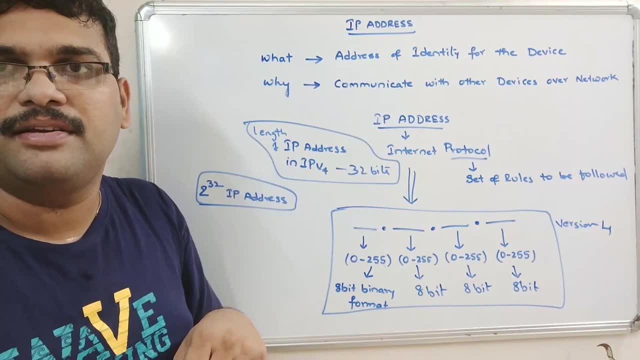 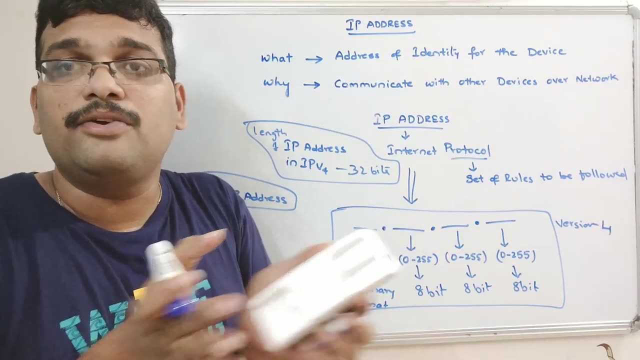 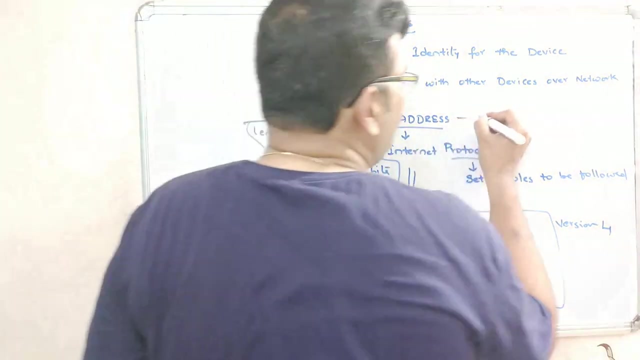 Right, So no, two systems must have the same IP address. So if two systems are having the same IP address, automatically that data will be sending to both the systems, Right? So the IP address should be unique. Okay, This IP address should be unique. 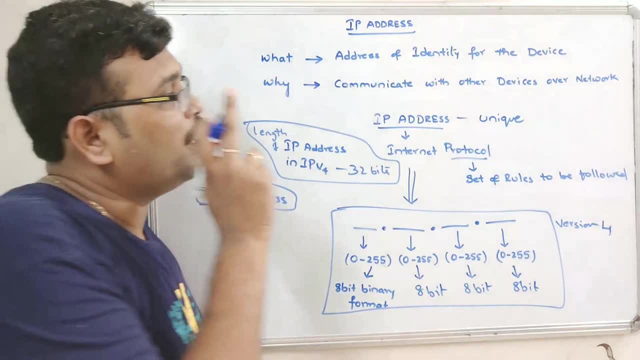 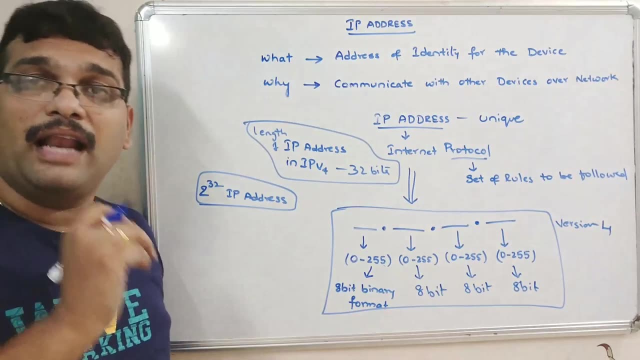 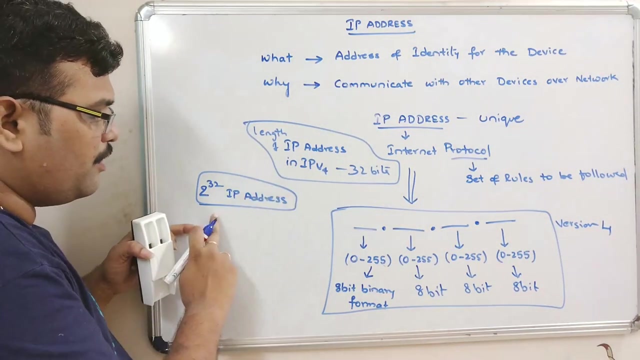 It should not be shared with any other system. Right, So, one IP address to the one device it has. Either it may be mobile or it may be a tab, or it may be computer Or it may be laptop. Right So in the IP version 4, the IP addresses can be generated to 2 power, 32 devices. 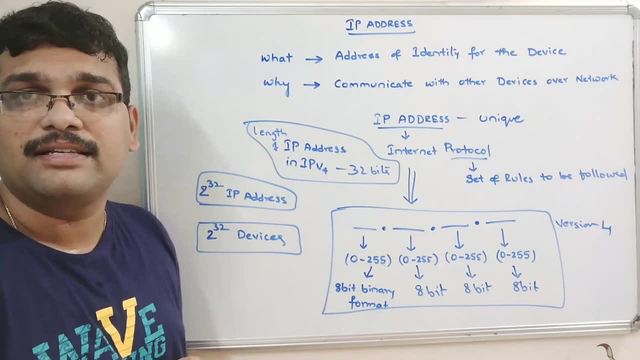 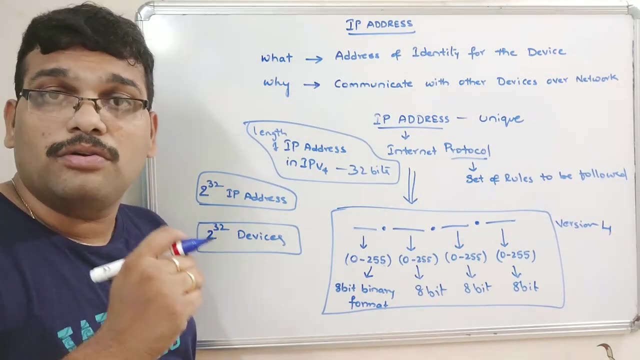 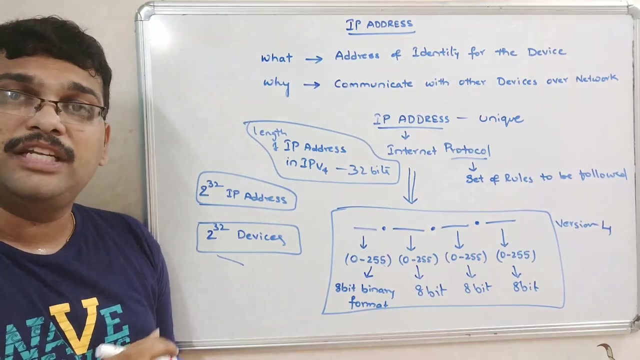 2 power 32 devices. Only 2 power 32 devices, So, but nowadays we know that everyone is having a mobile phone And also the computer or a laptop or a tab, So automatically This will give- this will be- a shortage of IP addresses. 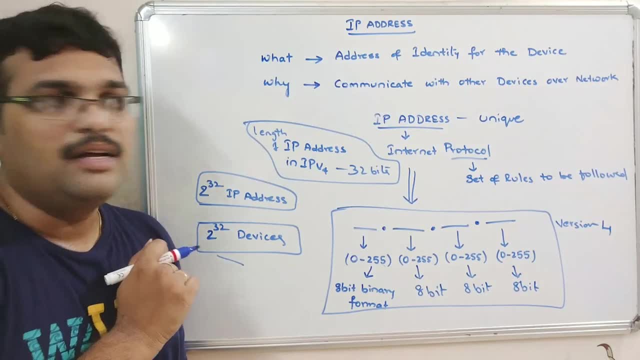 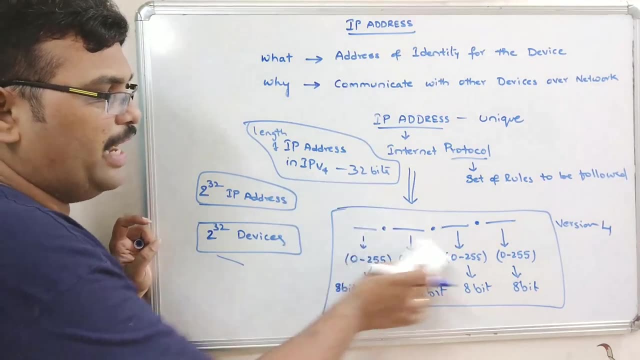 Right, This number is obviously a shortage of IP addresses, So that's why we are moving on to the IP version 6.. Right, So this is all about version 4.. So 8 bits will be there Now. 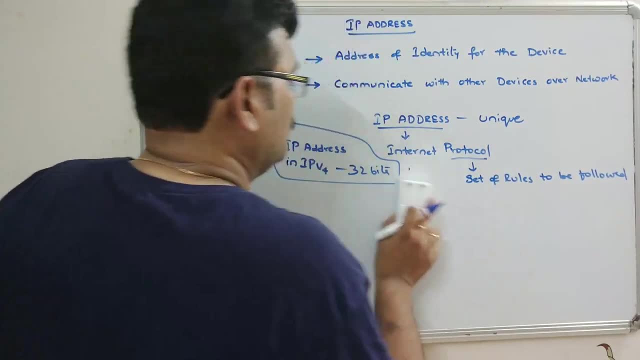 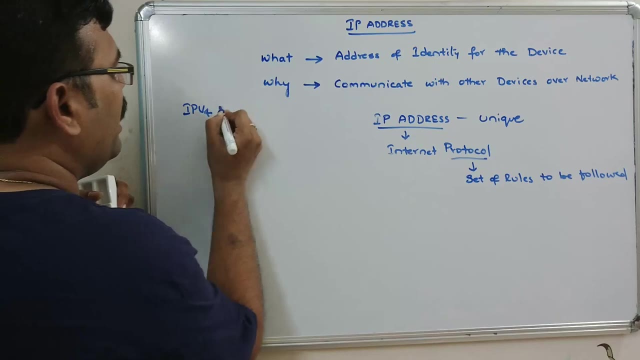 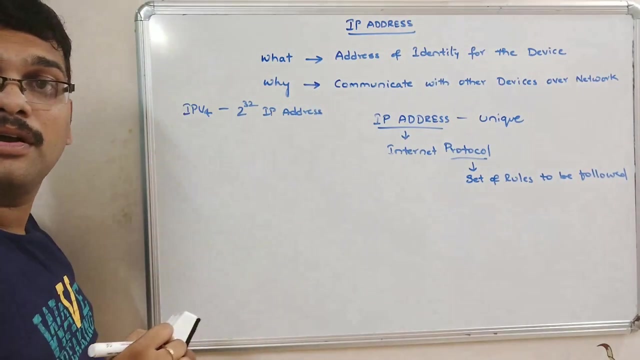 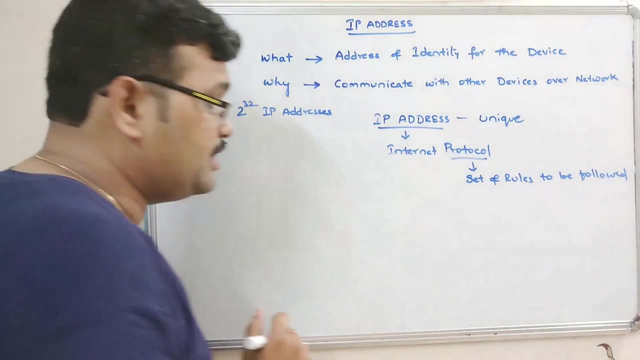 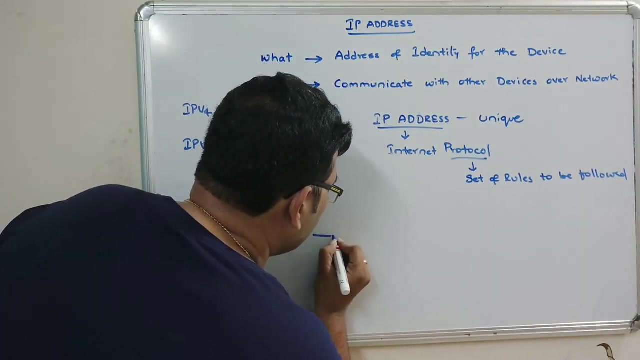 Now See. So only IP version 4 can have 2 power 32. IP addresses: Okay, IP addresses, Now IP version 4. Sorry, IP version 6. IP version 6.. So there are 8 parts separated with dock. 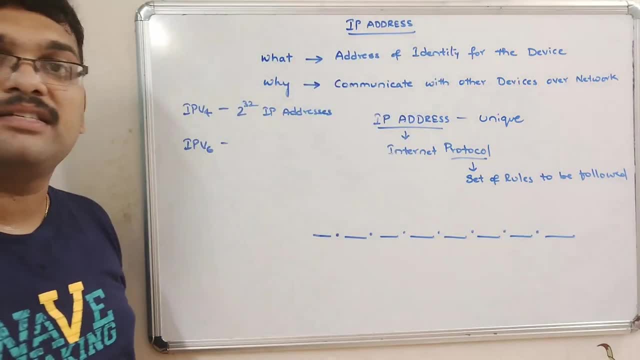 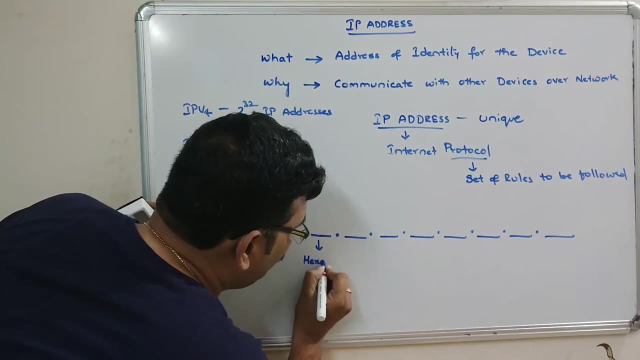 1,, 2,, 3, 4.. 1,, 2,, 3,, 4,, 5,, 6,, 7,, 8.. 8 parts separated with the dock And every part will be fixed with hexadecimal format. 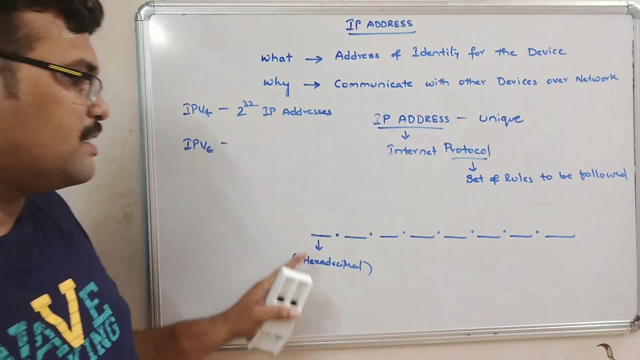 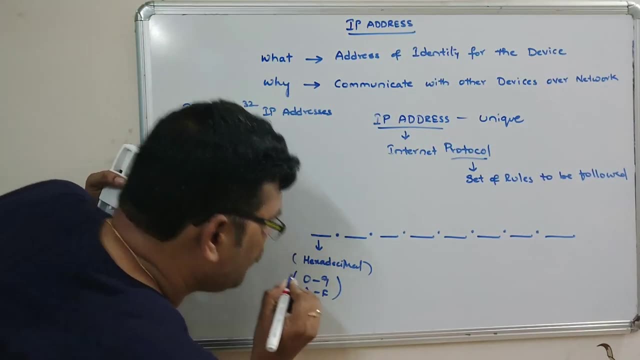 Hexadecimal, So every part will be filled with hexadecimal. We know that hexadecimal are nothing but 0 to 9 and A to F, Combination of 0 to 9 and A to F, Right, So hexadecimal Every column. 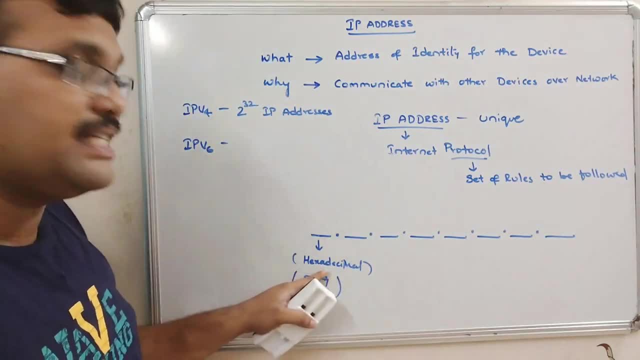 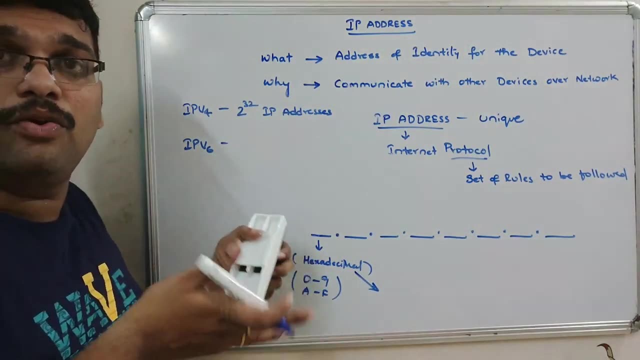 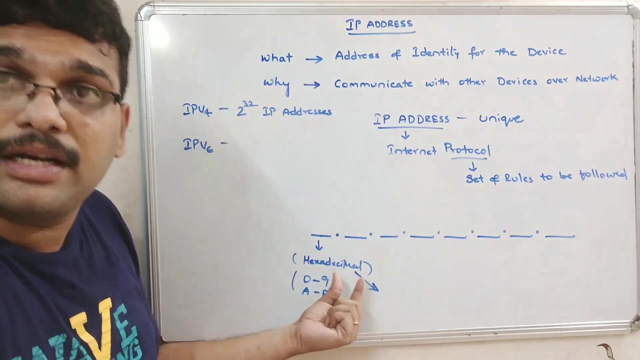 I mean every section will be filled with hexadecimal format, Right? So if you convert this hexadecimal format into binary equivalent- Because the system only knows about the binary formats Right- Either 0s or 1s- So if this hexadecimal format is converted into binary, it must be represented using 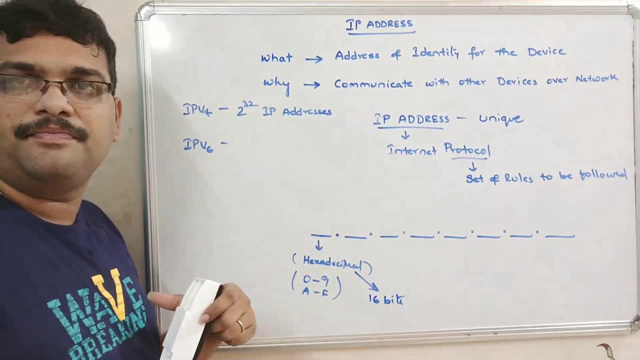 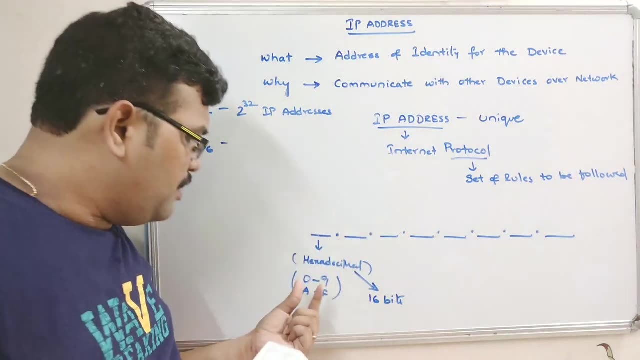 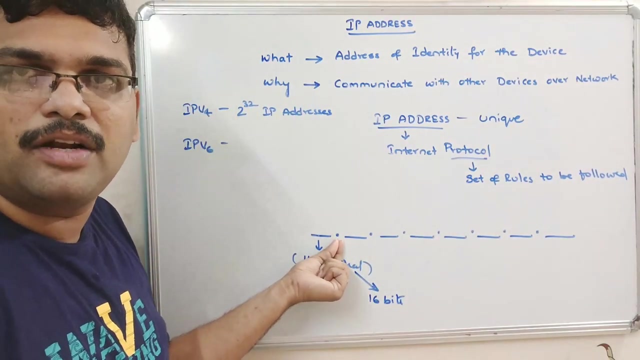 16 bits, 16 bits, Okay. So if you observe any IP version 6 IP address, you can know the combination of numbers and alphabets with 8 sections. 8 sections divided with dot, Separated with a dot. 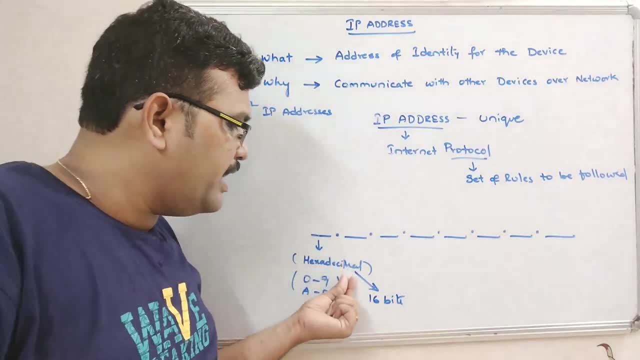 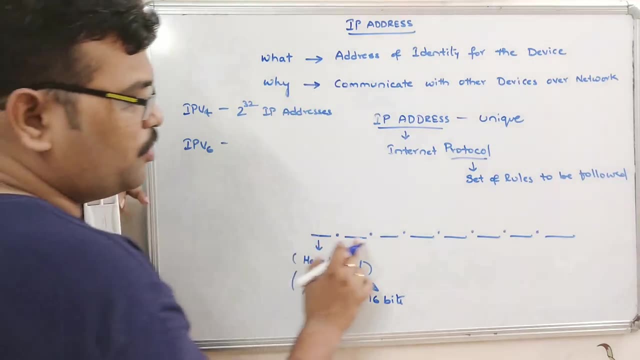 So that is nothing but a hexadecimal separated with a dot, And this hexadecimal is represented in 16 bits, 16 bits. So this 16 bits total 8 into 16 bits, So this will be again 16.. 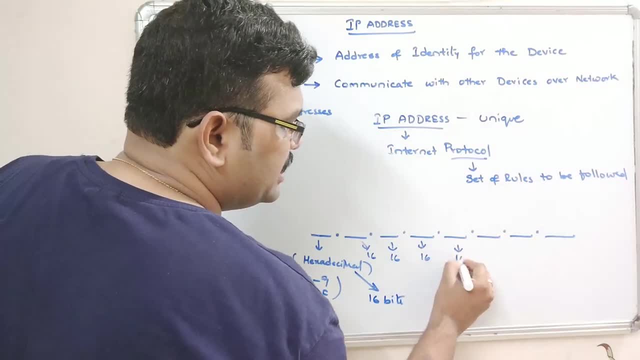 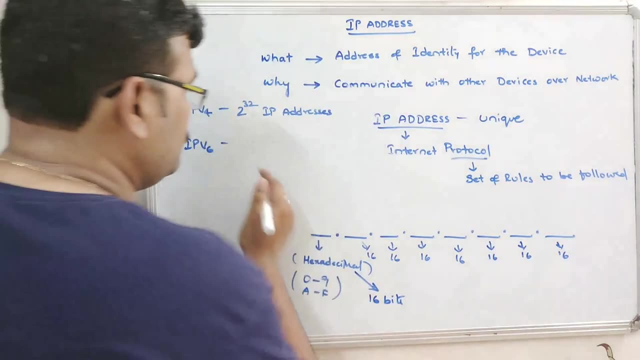 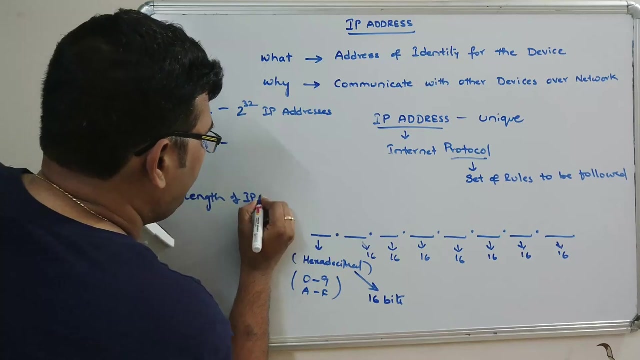 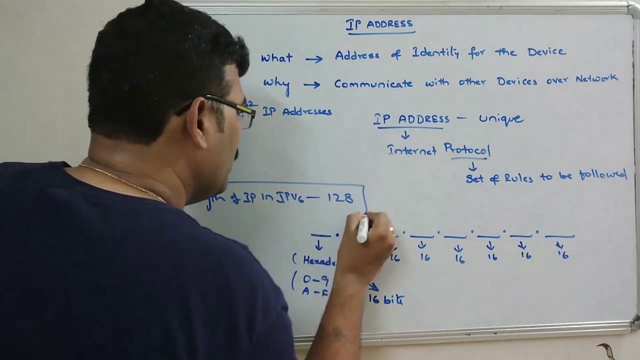 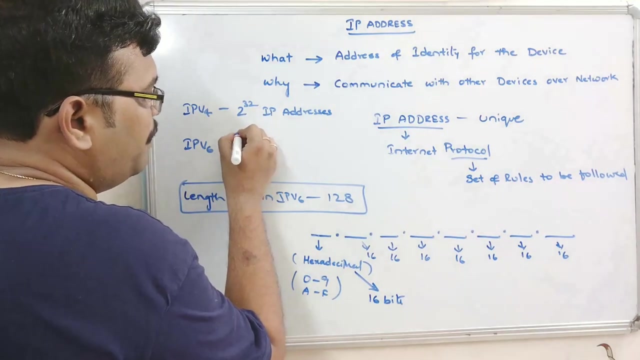 This is 16.. This is 16.. Again 16 bits, 16 bits Right, So 8 into 16.. So total length of IP in IP version 6 is 128.. 128. So that from the IP version 6, we can generate 2 power, 128 IP addresses. 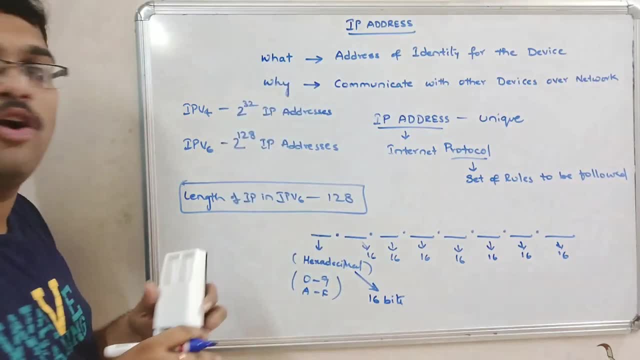 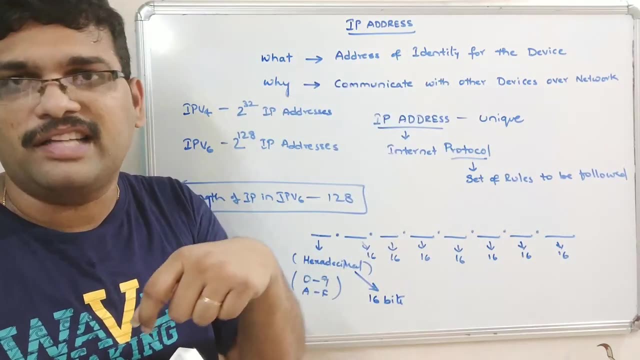 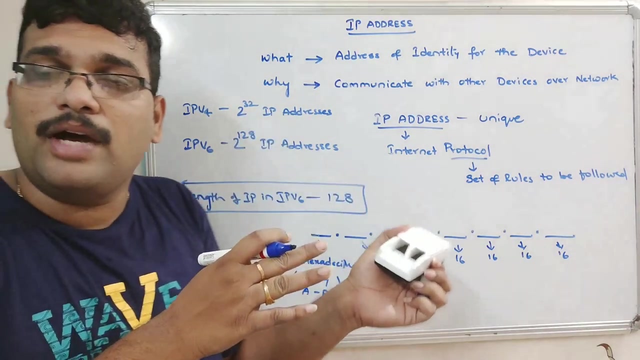 So that means we can accommodate Around 2 power 128. Around 2 power 128 IP addresses, So that devices may be the mobile, laptop or desktop, as I have said earlier. Right, So this is the reason why we are moving from IP version 4 to IP version 6.. 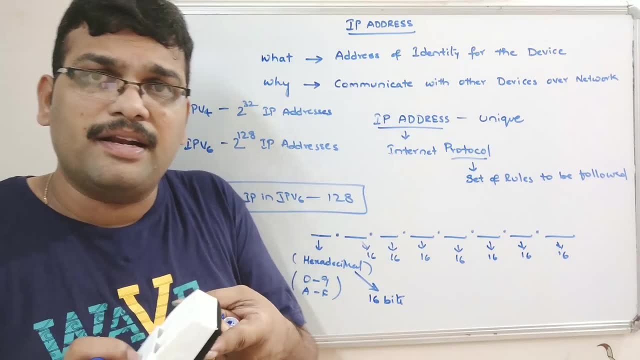 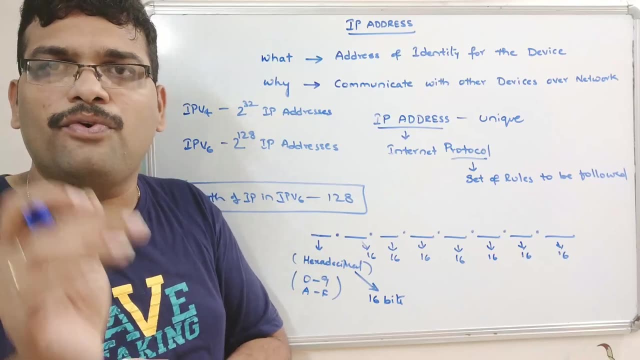 So just one thing. So if just find out the IP address, So you can go to Google search and you can type what is my IP address, So that it will give your particular phone or a mobile- I mean systems- IP address. 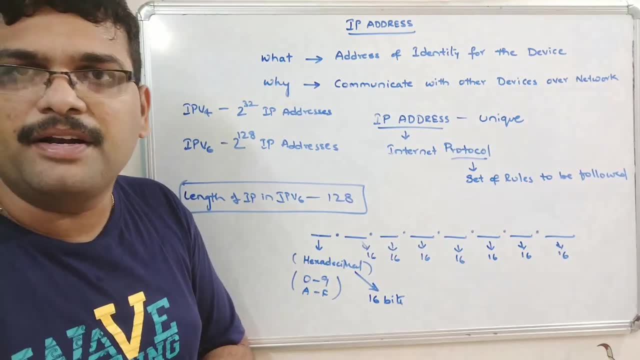 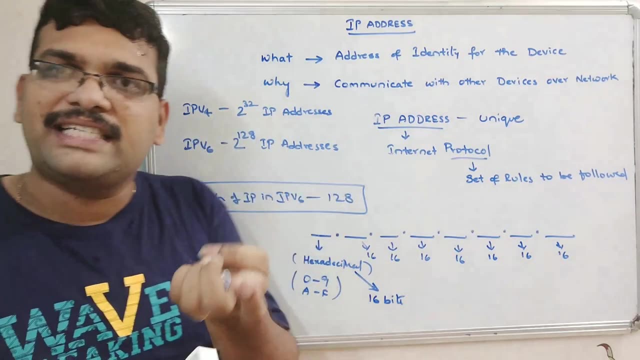 It will give Give result as your IP address Right, Which IP address you are having. So you can observe that if it is a version 4, the 4 sections will be there. The numbers will be in between 0 to 255.. 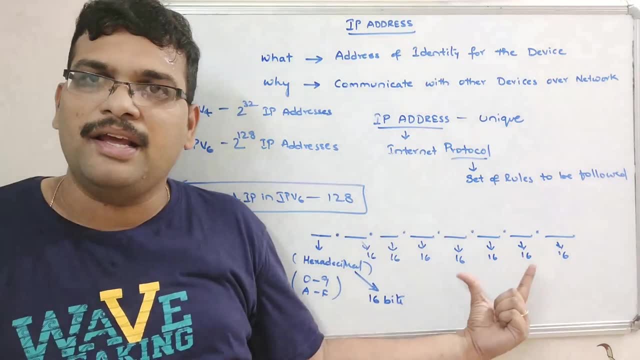 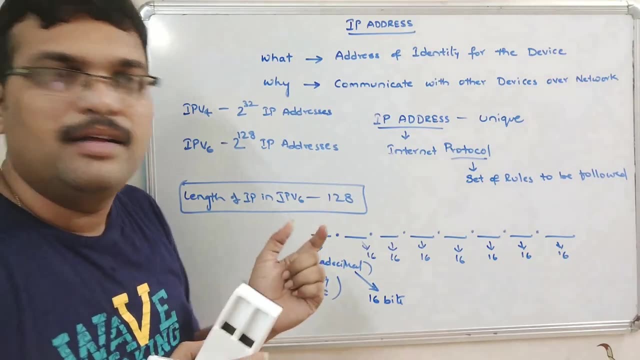 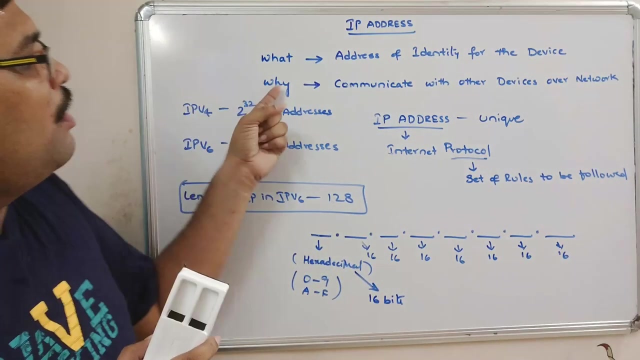 And if it is IP version 6, 8 sections will be there And each section you can find the hexadecimal formats, Hexadecimal numbers, Right. So hope you understood this simple introduction to this IP address. So what is IP address and why we are using this IP address? 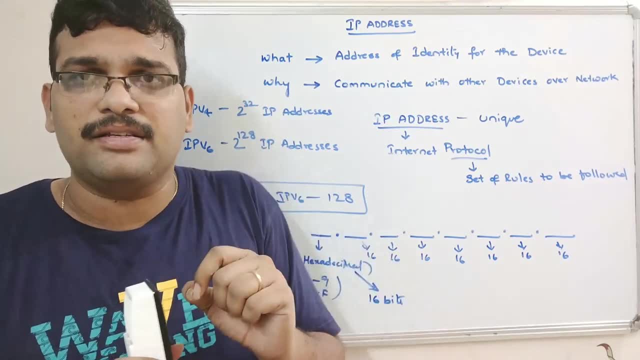 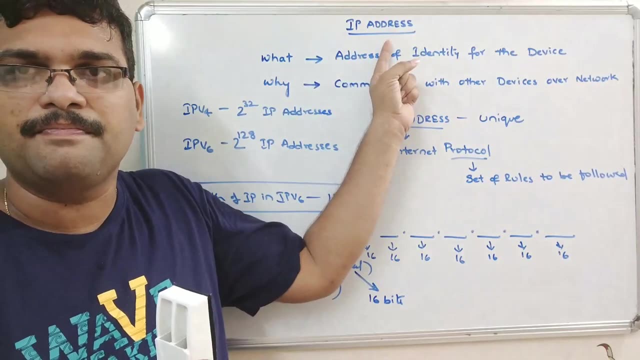 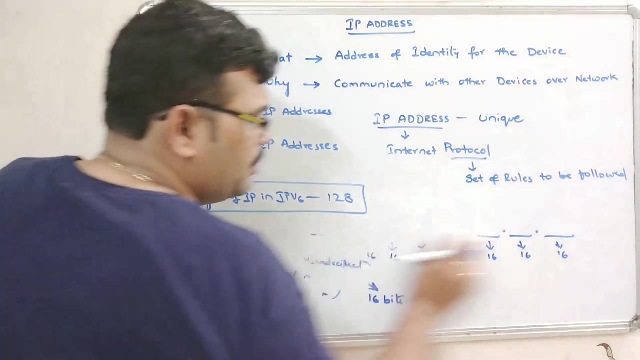 So every device should have an unique IP address. So, in order to communicate one device to another device, that will be done only by the means of this IP address. So so, everything there will be having an IP address, But so whatever we are typing in this URL. 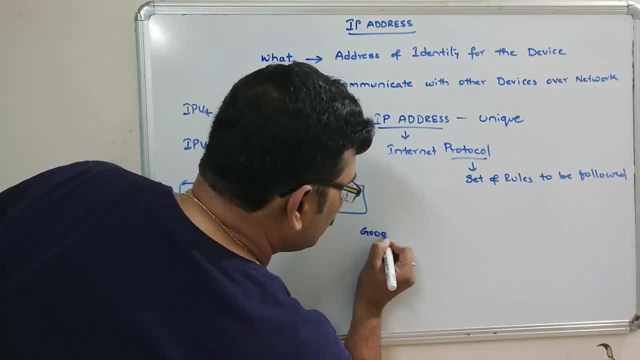 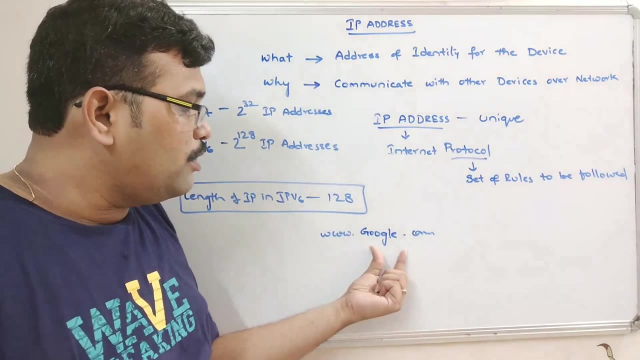 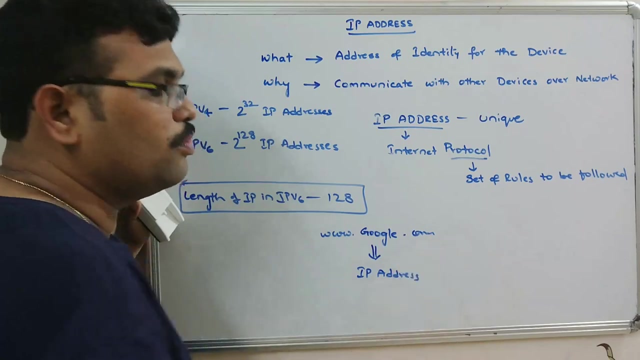 See, for example, we are going with a googlecom- Right Right, Right, wwwgooglecom. So actually this googlecom will be converted into IP address because the system does not know this google and all these things. So system only knows the IP addresses. 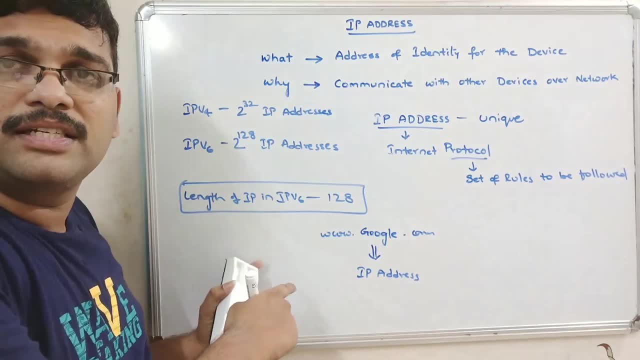 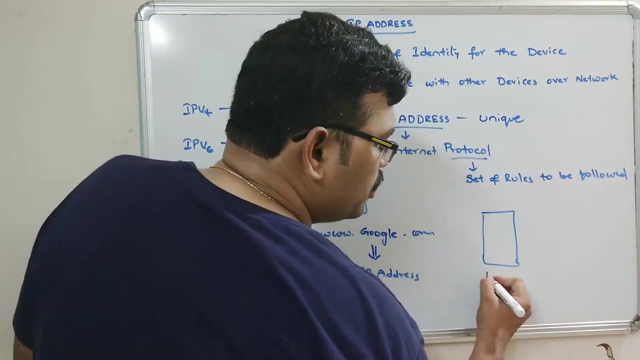 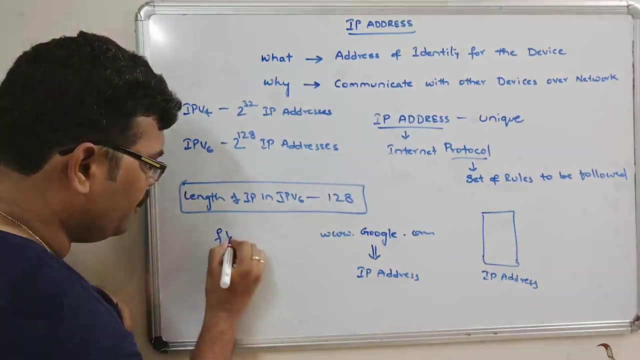 So IP addresses means IP version 4 or version 6. So every device will be having the IP address. So here a google server will be maintained and this google server will be also having some IP address. So So, similarly, if you go with the e-commerce websites- some flipkart, flipkartcom or amazoncom- 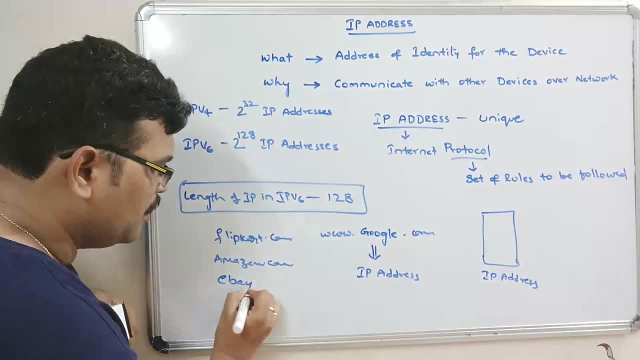 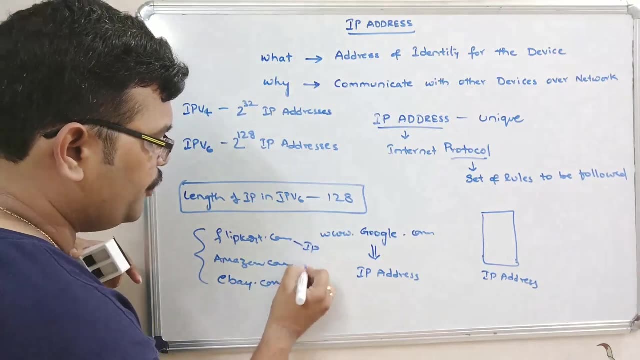 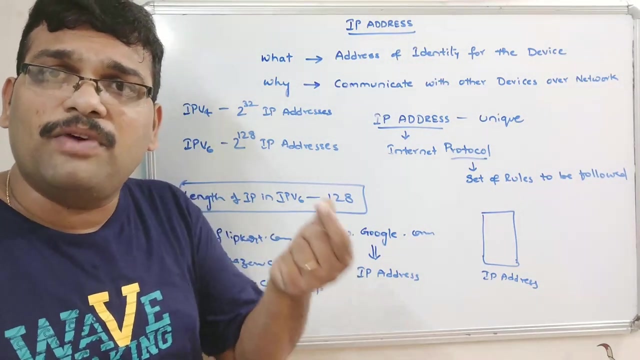 Right. So similarly ebaycom. So for every website, for every website, for every website, there will be some IP, unique IP Right, Right. So for an user it is somewhat difficult to remember All these websites with the help of this IP right, because IP will be having four sections. 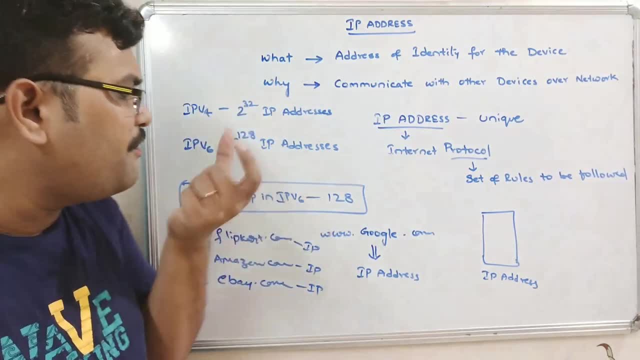 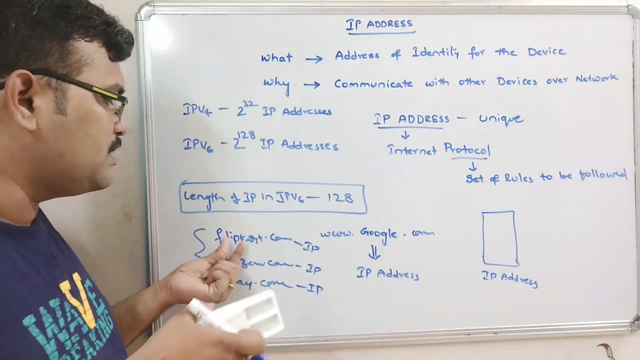 with different numerical terms, right. So it is somewhat difficult to remember these numerical IP address for the user. So we are converting this IP into some domain name. So this flipkart is a domain name, Amazon is a domain name. 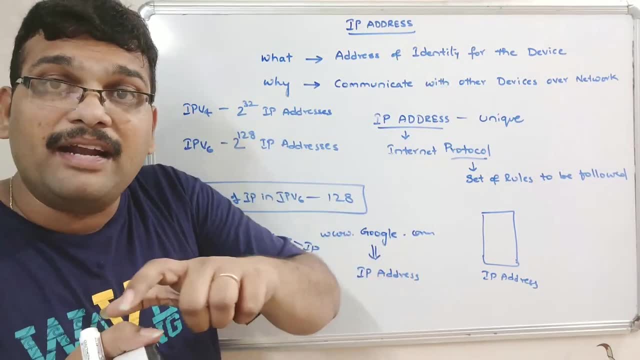 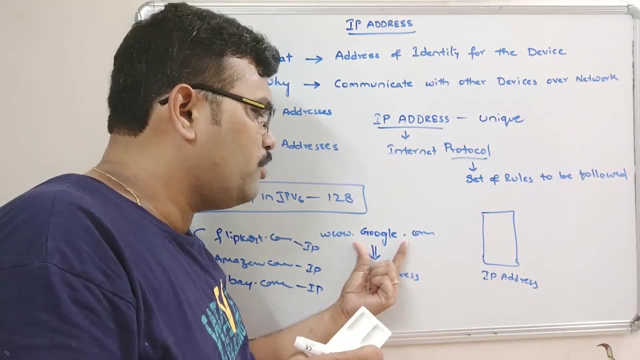 eBay is a domain name, Google is a domain name, So the IP address will be converted into domain name so that we can remember the domain names. and if you enter- So if you enter this wwwgooglecom, immediately that domain will be converted into IP address. 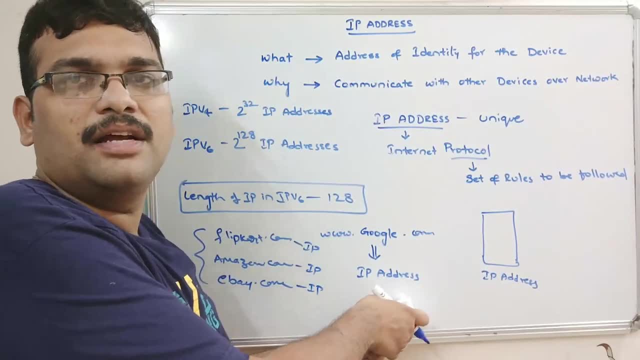 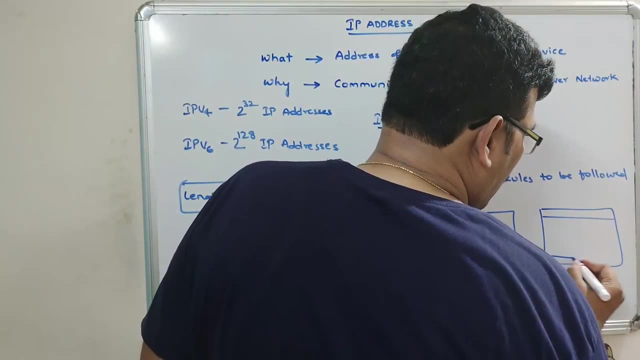 and then the request will be sent to this IP address. So you can find this IP address at the bottom left of your web page. So at bottom web page of your- I mean bottom left of your web page- here you can find the. 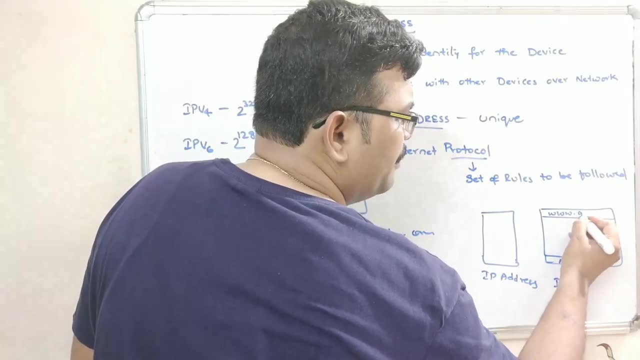 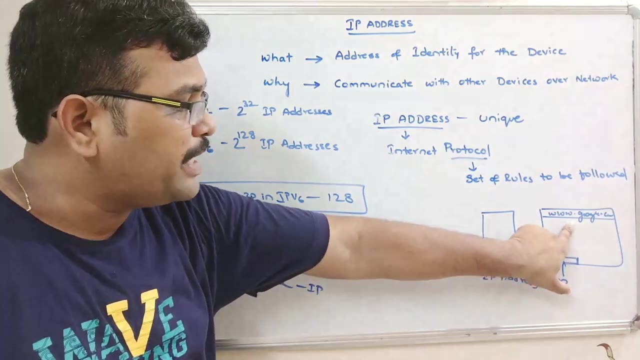 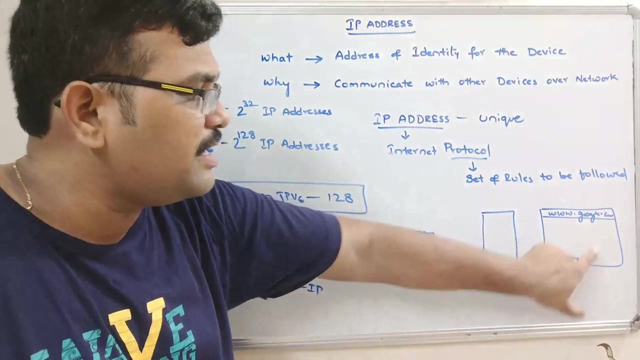 IP. if you type this googlecom, So whatever it may be, Not only the googlecom- whatever the website you are entering, So whatever the website you are typing, that particular IP address will be converted. I mean, this domain will be converted to the particular IP address and the request will. 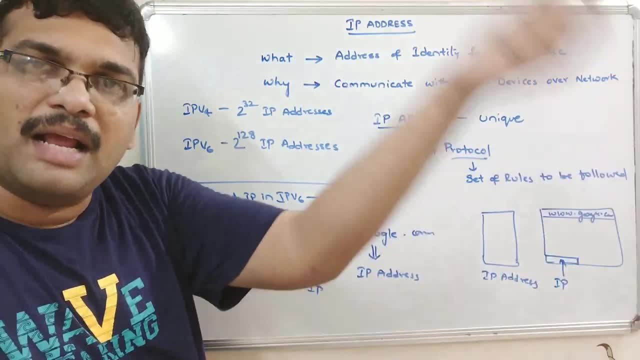 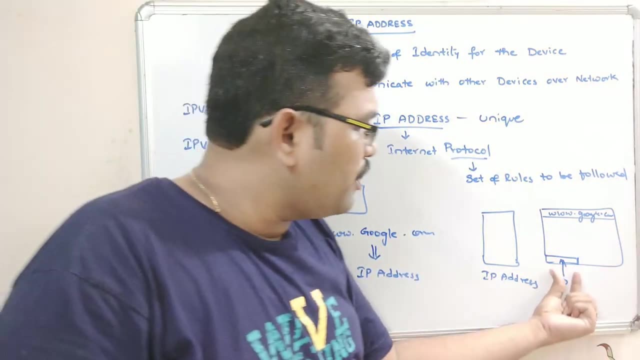 be sent to that particular IP address. Similarly, that particular IP address, that response will again send to the same IP address from which it accepts the request, right? So here you can find this IP address. It will be a fraction of seconds. 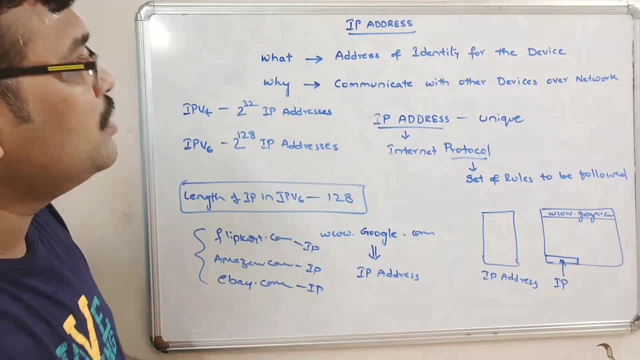 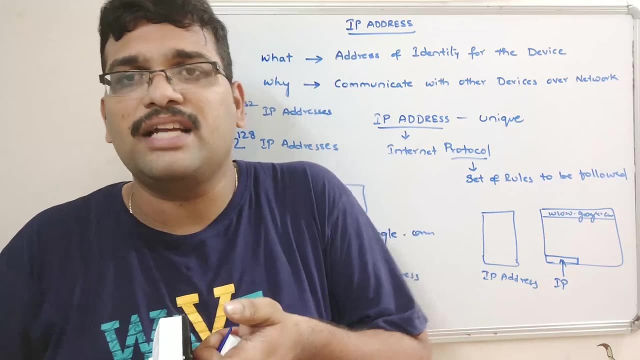 So once you find out, so you can know about these IP addresses, Right? So hope you understood this. So what is the IP address and why we are using this IP address? Only one answer for why you are using is communicating with other devices over network. 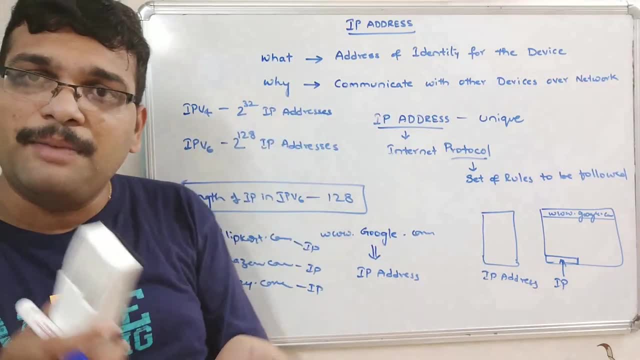 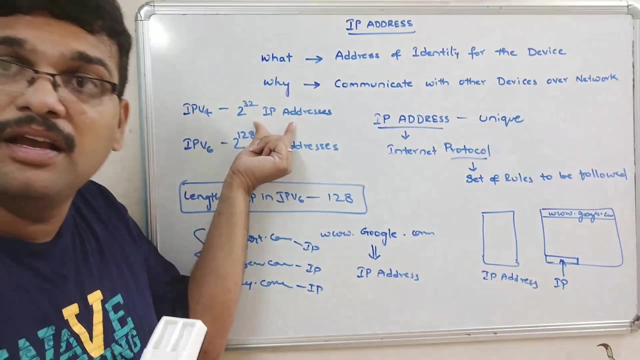 Right. So in this session we have seen IP address, the length of the IP address in version 4 and version 6.. So in the version 4, there is a drawback that only limited number of devices can be. I mean IP. 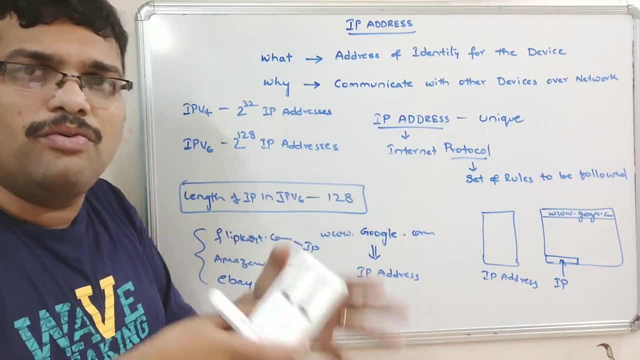 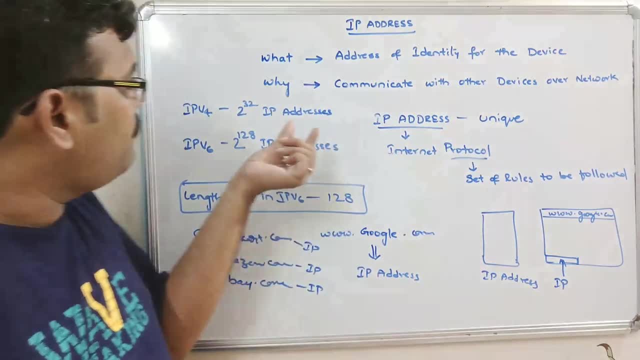 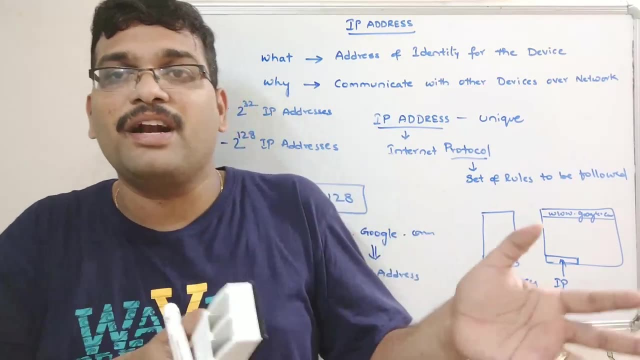 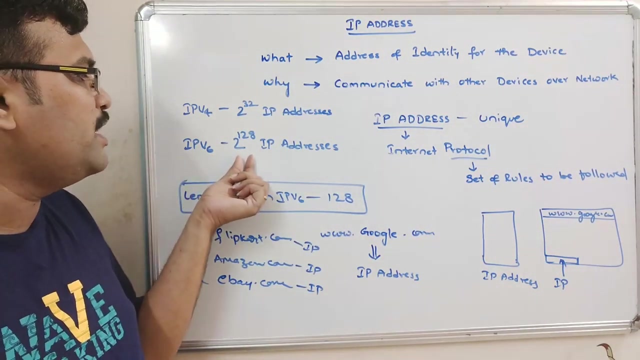 So this is not sufficient to accommodate all devices. For that purpose, we are moving to the IP version 6, which is represented as a hexadecimal format in 8 sections separated with a dot Right. So the length of the IP address in version 6 is 128.. 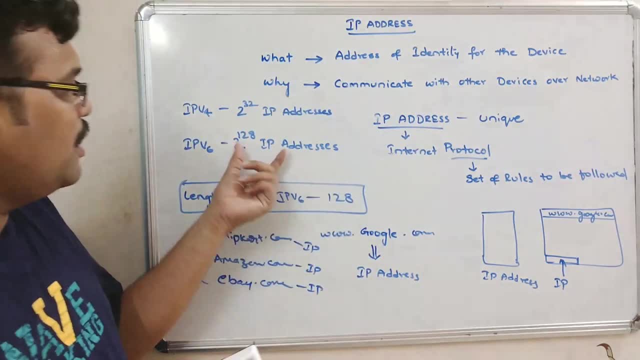 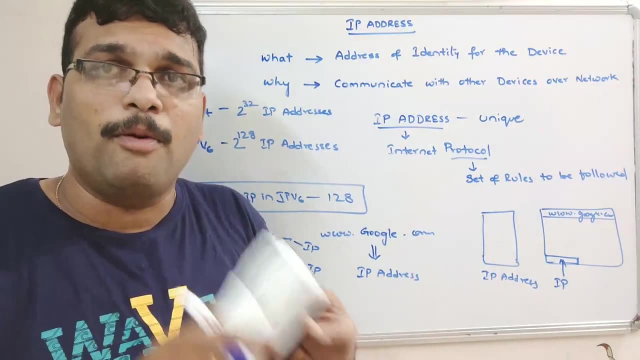 So 2 power 128 devices can be accommodated by giving the unique IP addresses. So for every device there must be one unique IP address, Either it may be a laptop or a mobile data system or system desktop or a tablet. 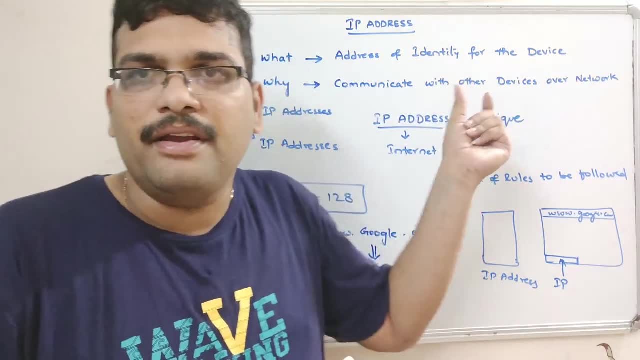 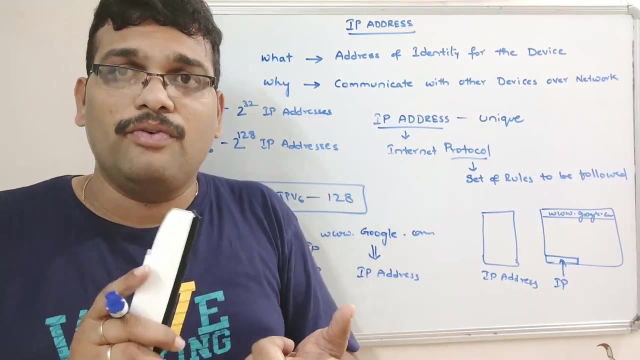 So, whatever it may be, there will be some unique IP address So you can find by typing what is my IP address in Google search. So whatever device you are using, either mobile or desktop or a laptop- just type what is my IP address. 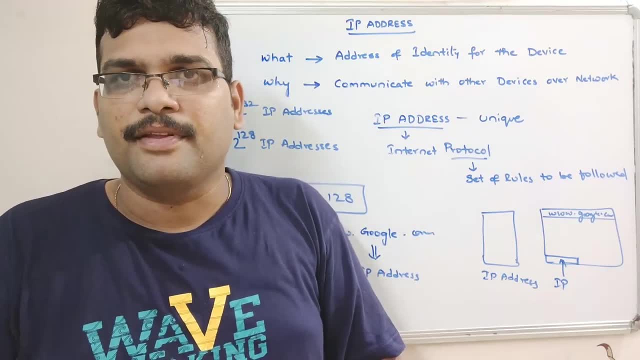 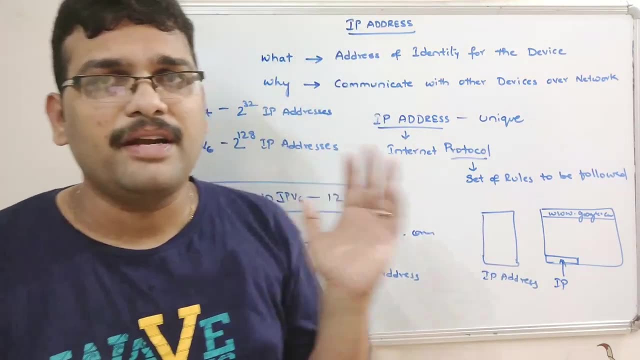 So it will give the IP address of your particular device, Alright, So let us stop here. I hope you understood and enjoyed the session. Okay, Okay, Okay, Okay, Okay. doubts regarding this ip address. so feel free to post your doubts in the comment section so that 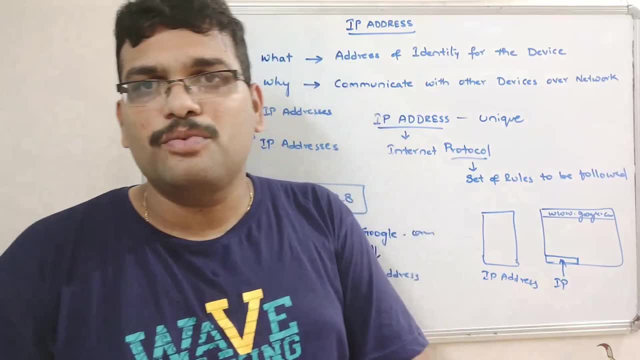 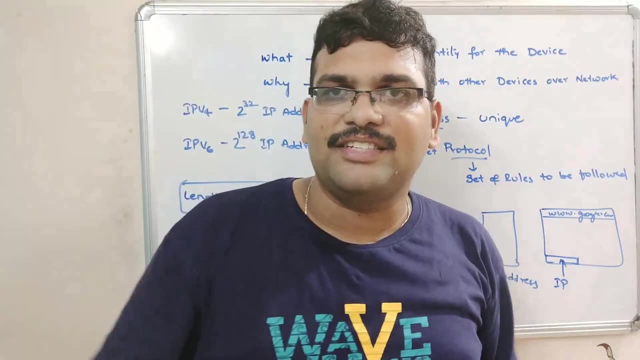 definitely. i will try to clarify all your doubts and if you really understood my session like my session, share my session with your friends and don't forget to subscribe to our channel. so thanks for watching. thank you very much.